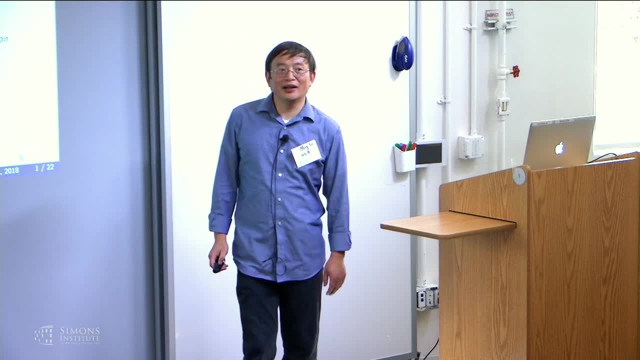 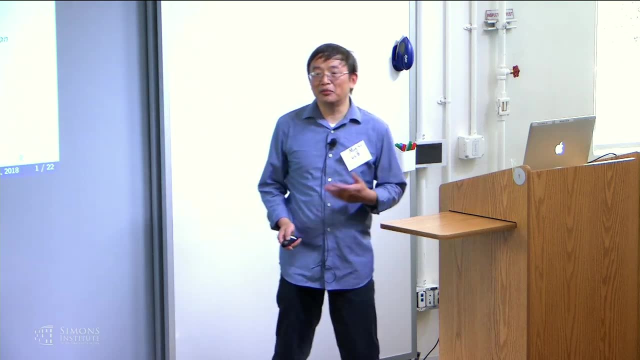 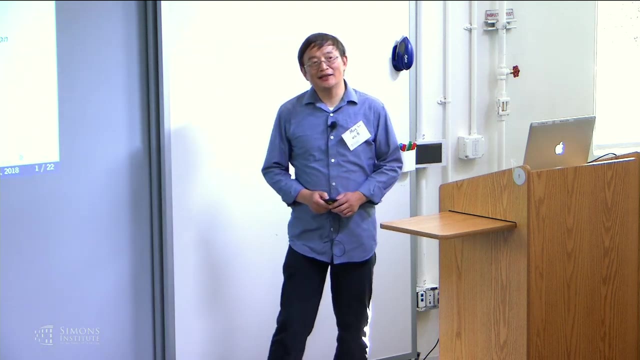 This is what we've been doing over the last few years and most of the people here they are graduate students. Some of them are still here. Some of them have graduated. So Dave Anderson, he's at Google now. Jay Josh, he's at the same year. 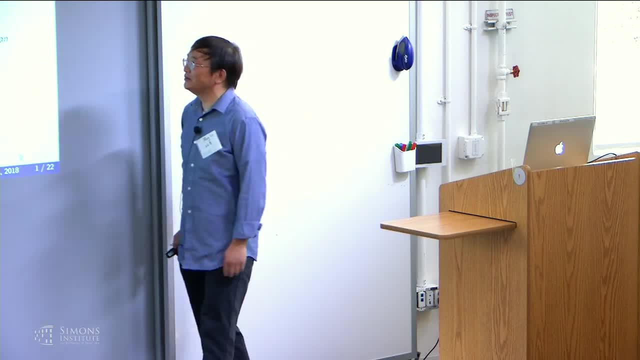 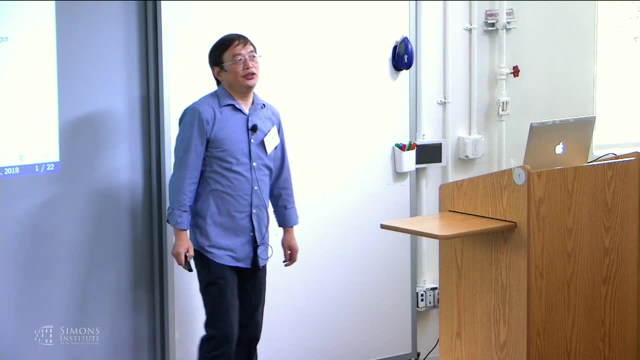 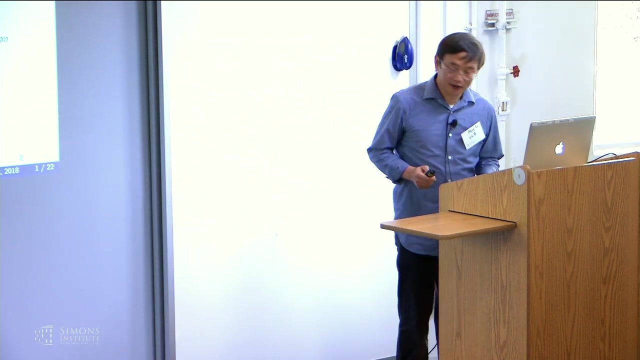 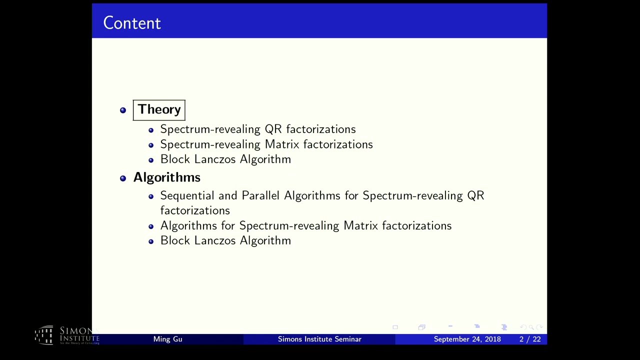 Eric Holman- he's still here. He should graduate next year. Bao Li is also here. Zhengwei Shao: he's actually going to Facebook. So is Chaozhu Yuan Contact. So this was supposed to be an hour talk, so I'm going to squeeze a lot of stuff and I'm going to skip a lot of material as well. 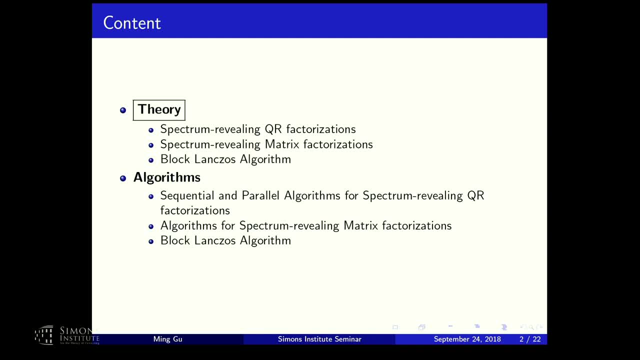 And Yusa already threatened me to cut me off if I go over 30 minutes, So I will mostly focus on the theory part of this And we're going to talk about what's called spectrum-revealing QR factorizations. Traditionally there's something called rank-revealing QR factorization. 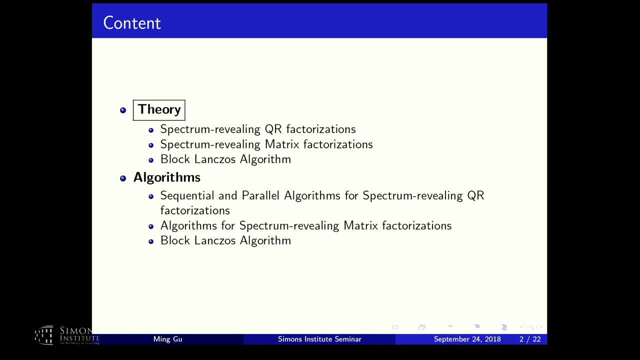 We're going to review that and see what the difference is. And we can generalize this idea to most of those matrix factorizations And get similar results. And we're also going to look at the blocked Lanczos algorithm. This is all for lowering approximations. 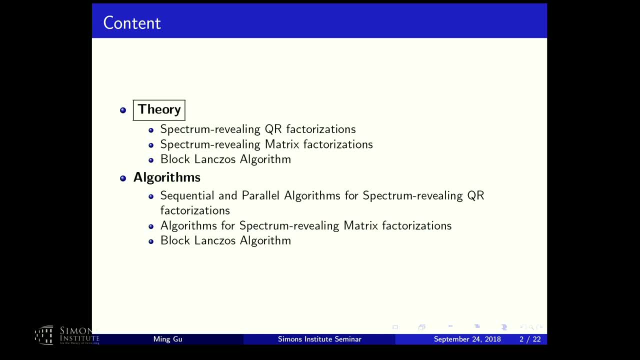 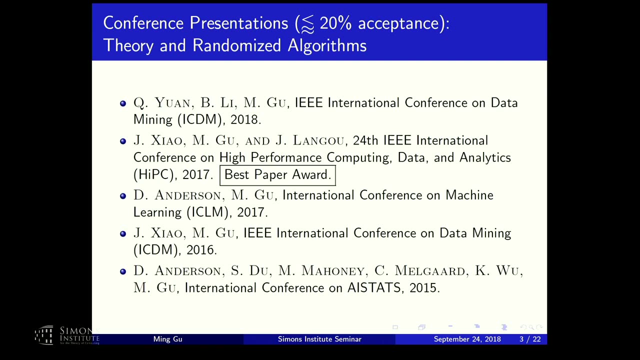 And there's a number of different methods that have been developed for these factorizations, And I'm going to, if I have time, focus on this QR part of this And I'm going to skip the rest of these things. So over the past few years, we have been submitting these papers. 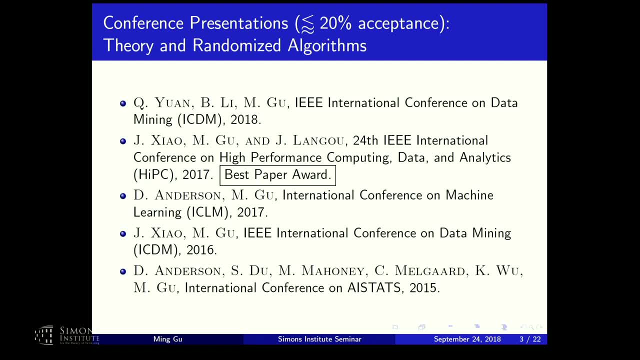 And we got so far five acceptances at these top machine learning conferences, And typically the acceptance rate is less than 20% And one of the papers received this best paper award. This was like in 2017,? I think Yes. 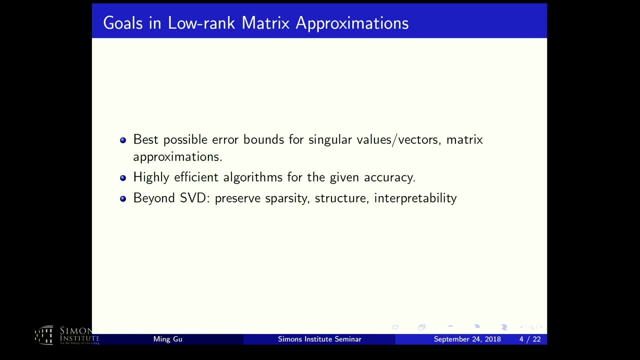 Okay, so what is going on? So we're trying to come up with, you know, for any given factorization, we try to get the best possible bounds And we try to find methods that can compute these factorizations efficiently And beyond low rank, as, like Mike Mahoney would say. 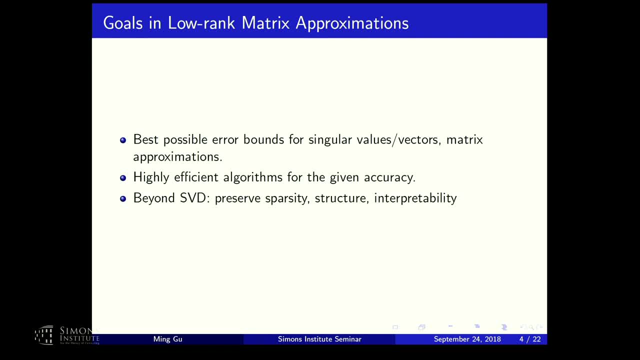 sometimes you can preserve sparsity or structure or maybe like in the column or in rows of the matrices, to get something beyond the SVDR. We're not getting into the details, but we're going to talk about some of these results if we have the time. 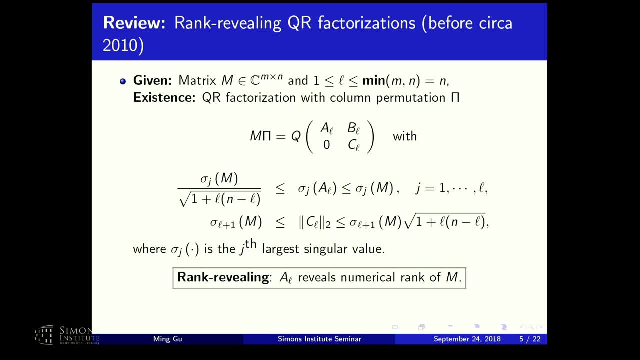 Okay, so this is the traditional way to look at rank-reading factorizations. So what you have is you're looking at a QR factorization, So here the Q would be orthogonal And this is going to be the R part of the matrix. 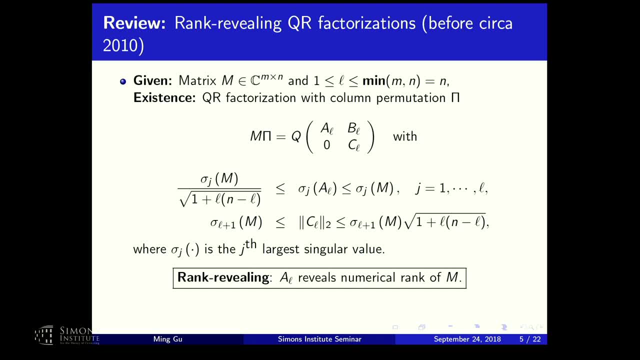 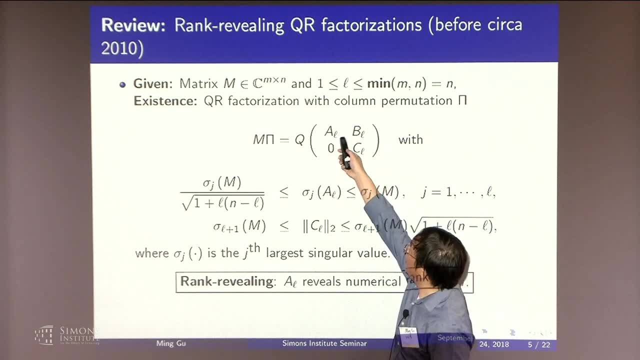 Pi is a permutation. So what you're doing is you're reshuffling the columns of a matrix M And after that you get a QR factorization. This can be a partial factorization up to this L. So traditionally, what we wanted to do was to figure out. 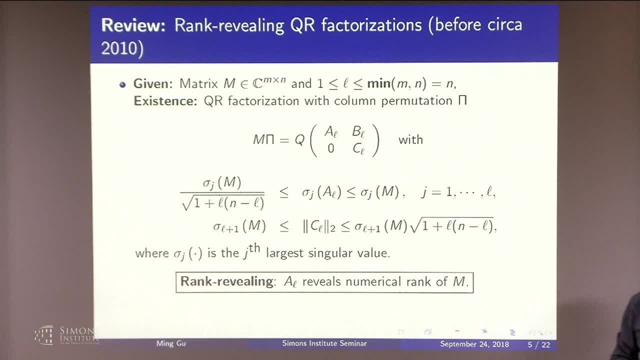 for example, the numerical rank of a matrix, so that you can do, for example, these squares correctly, And the focus is in finding the rank. So in this setup, what you can show is that you can find a permutation pi so that the leading piece, the L matrix, 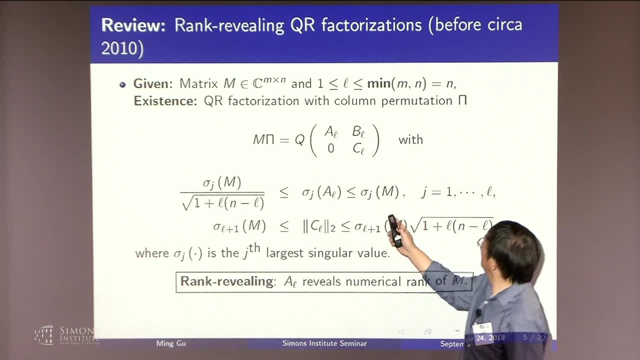 will have all its singular values 1 to L. The J would, So the primary G would be the J-th largest singular value. So all these singular values would match the original singular values up to a constant factor. Okay, so if you? 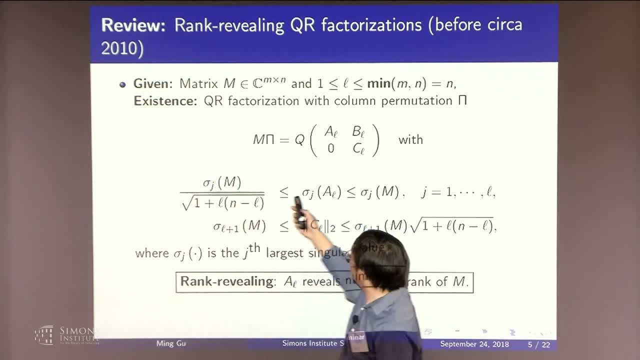 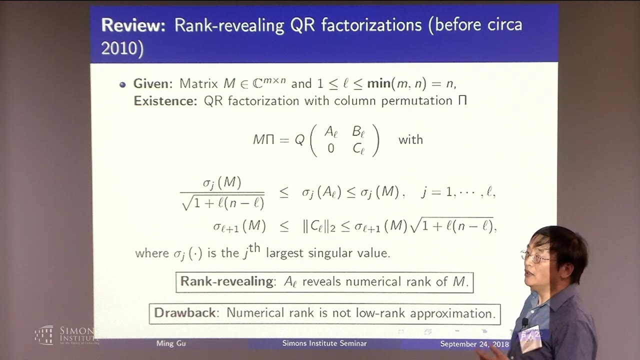 Let's say, the J-th singular value is tiny in the original matrix, this one would also be tiny. That would indicate rank deficiency. So that was the idea. So nowadays people do data analysis And what you want is a low-rank approximation. 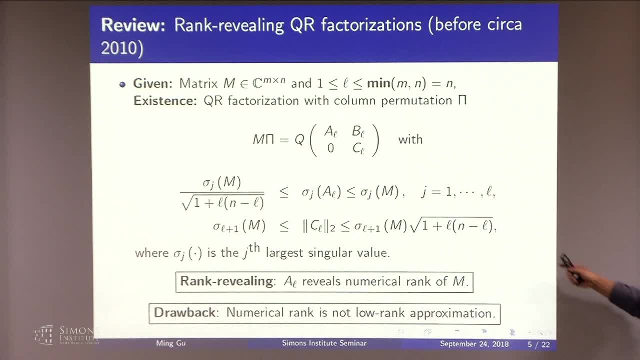 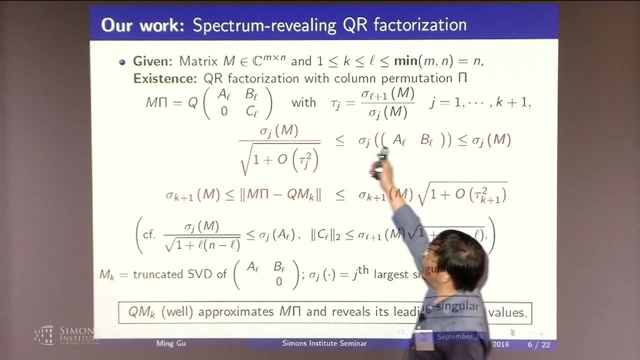 and not a rank determination. So this by itself does not tell you how you get a low-rank approximation or get it reliably. So that is the difference. So what we do is to look at it slightly differently. It's still the same: factorization. 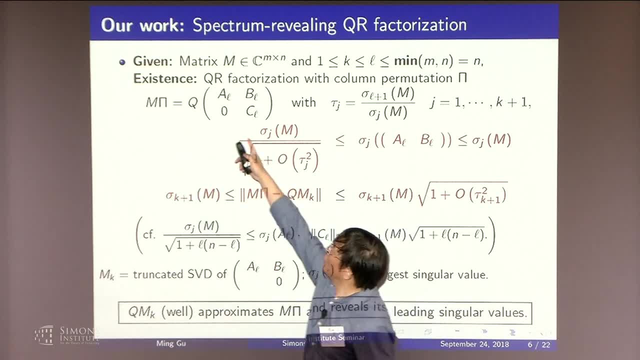 Again, this pi is the quantum permutation. You do a partial QR factorization, But what we're going to look at is not the matrix, AL Rather, it's going to be AL BL. You're going to throw away the CL part of the matrix. 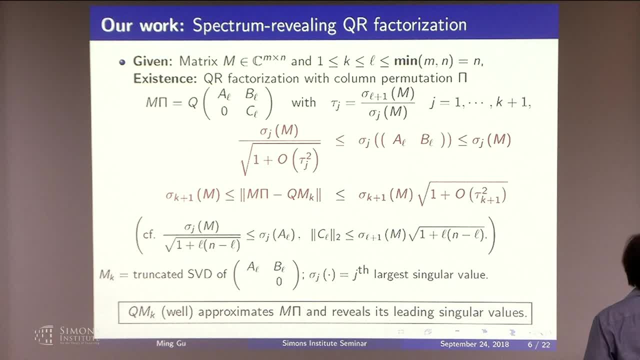 And now you do analysis. So if we define this tau J to be a ratio of these singular values, the L here is going to be the dimension of this AL matrix And the J would be the same index as the leading. It's the index of this leading singular value. 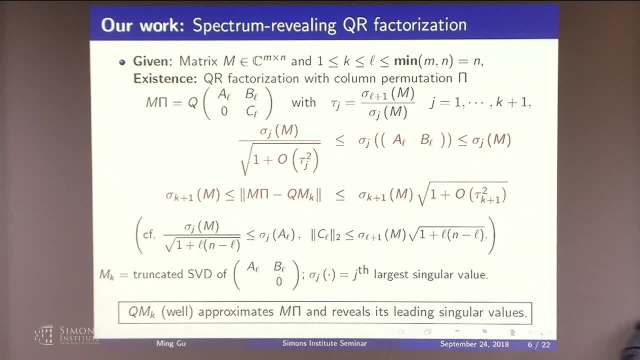 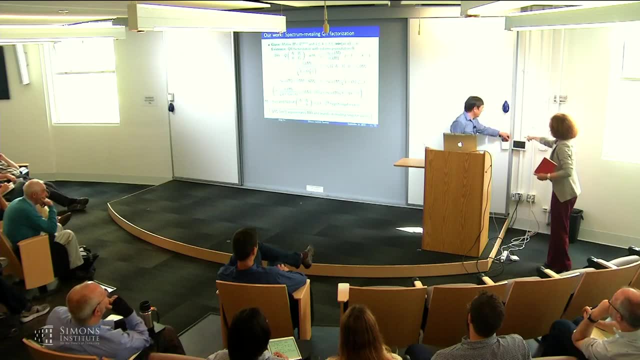 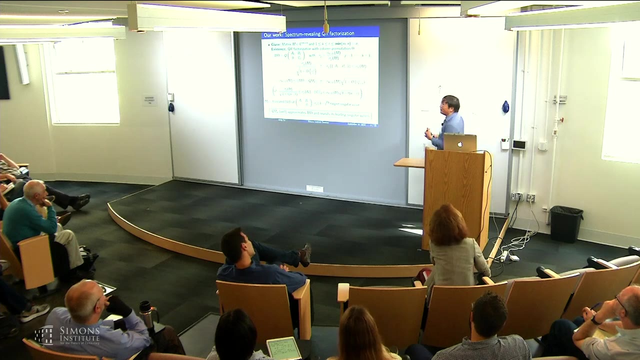 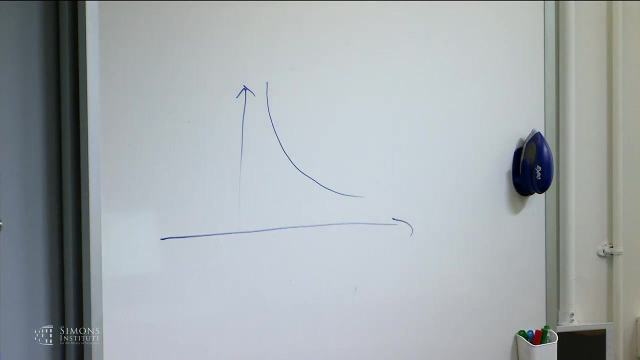 You take the ratio of this, what you would expect to get is this: Markers, Yeah, markers, Thank you. So, for example, typically you're looking at a data matrix, The singularities would decay like this, So there's no particular gap in the spectrum. 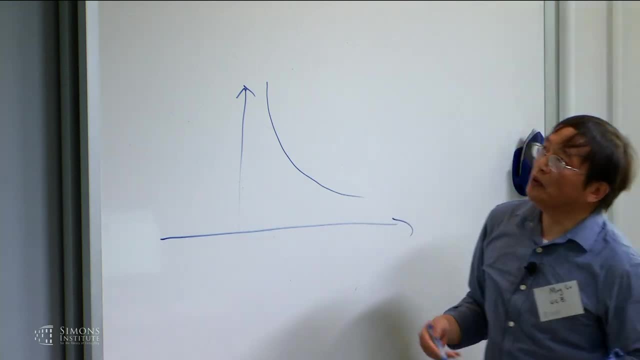 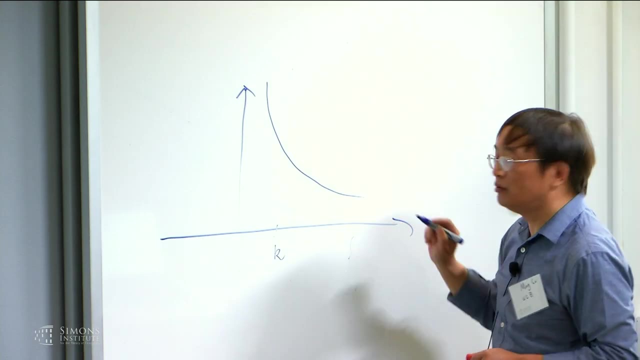 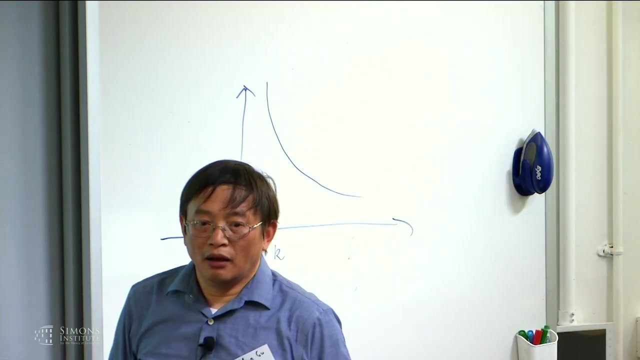 but singularities typically decay. So if you look for low-rank- let's say rank K- approximation, your K probably would be here And the L would be somewhere here, The G would be somewhere. Yes, Is AL not yet RL. 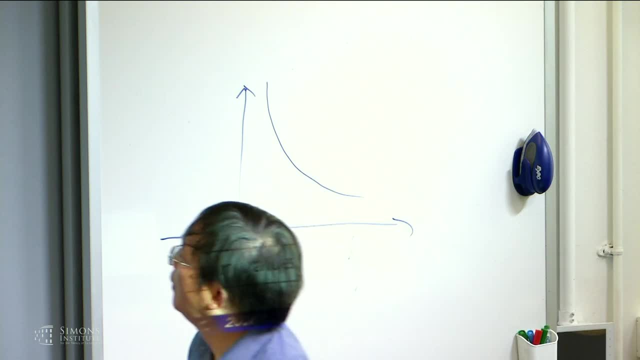 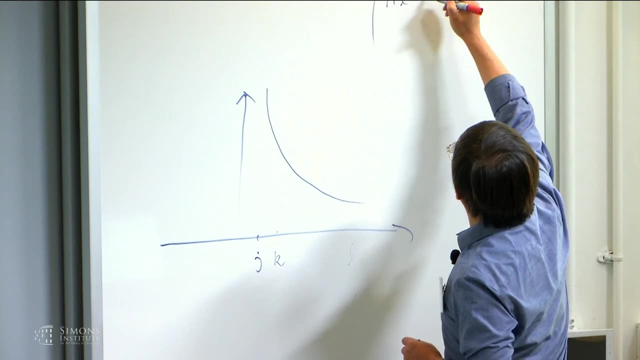 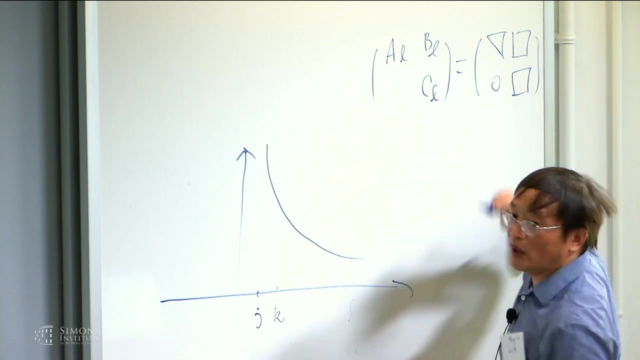 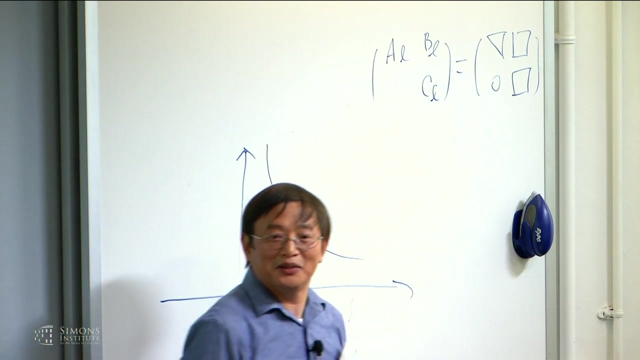 Is that AL not upper triangular? AL would be So the So why is it not RL? It would be typically like this What I'm saying: why not call it capital R? Yeah, maybe that would be a better notation. yeah. 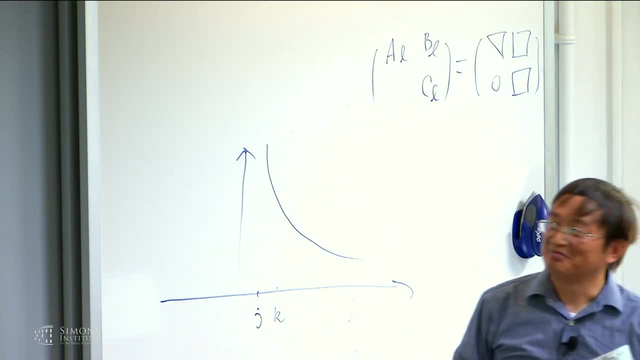 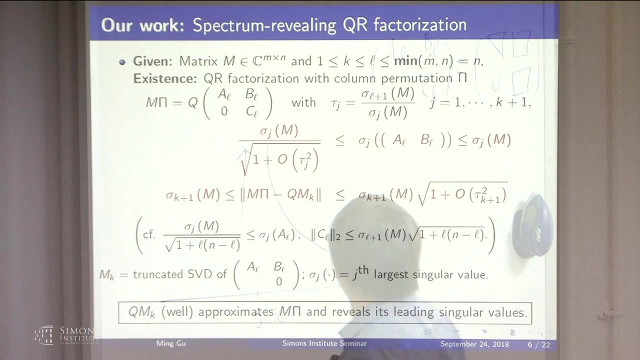 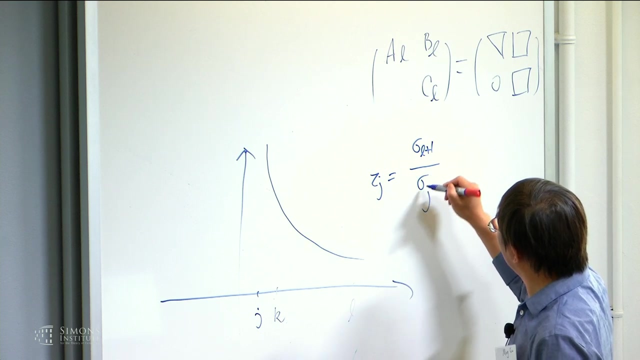 In the paper, in your paper, original paper- it's A right, We just didn't change the notation, sorry, Anyway. so we're looking at this tall J ratio, which is going to be sigma L plus 1 over sigma J. 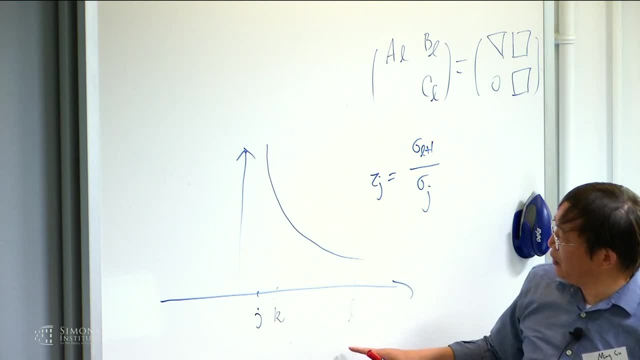 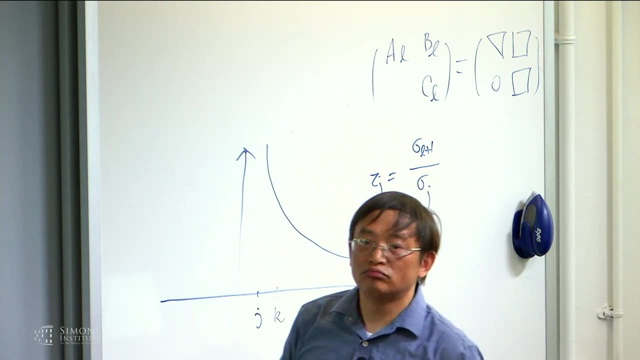 And you see that if you have a gap in between K and L, then you would expect this ratio to be reasonably small. Okay, It's not zero, but hopefully it's reasonably small. so that's why we actually We'll get to that. 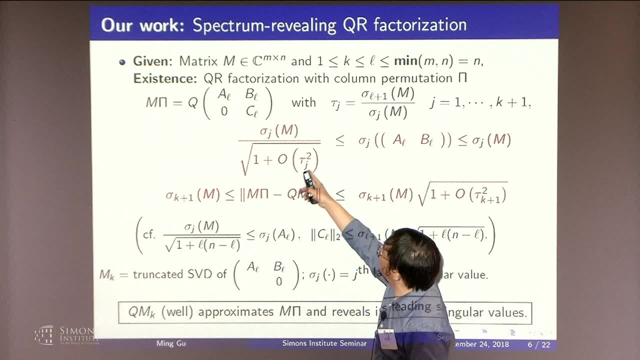 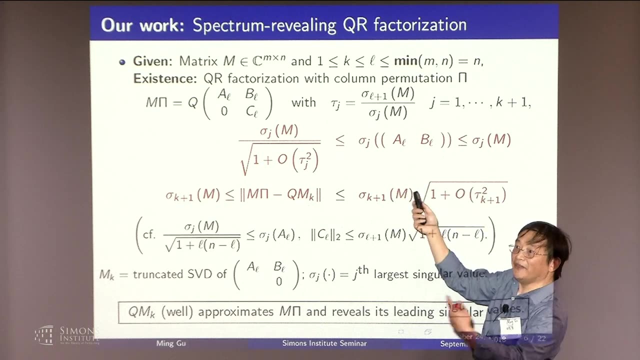 We hope that if this is small, then we can hope for this to be reasonably small as well. So if you're looking at this A or B or part of the matrix, then this matrix- not this one, but this one- will have leading singular values. 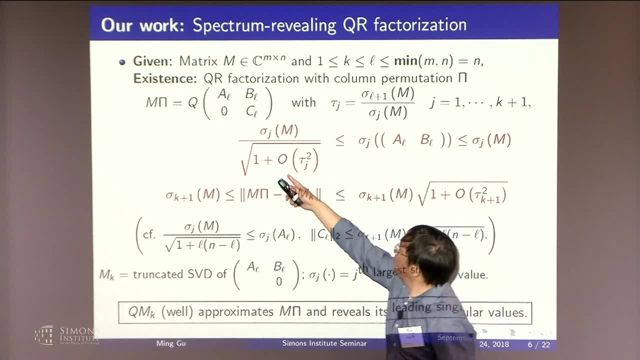 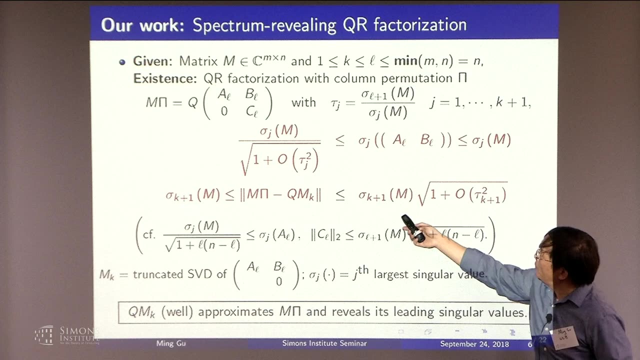 that are a close match to the original singular values up to this factor. Typically you would expect this to be small- Not always, but typically that's the case- And if you want to do a low rank K approximation then the error bound would be bounded below and above. 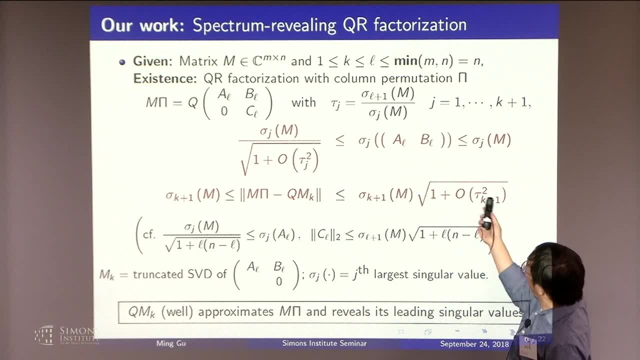 by these things and the only, The only thing extra would be this: Again, this is a tall dependent constant. so you have K plus 1. The K is the rank. So if you have a case where your singular values decay quickly, 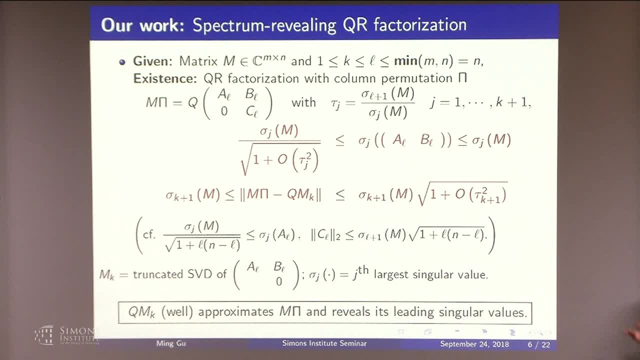 then even the tall K plus 1 could be very small. In that case, you would get a very good approximation, despite the fact that you're only doing QR factorization. Okay, This is different than the previous result in that here you only have a constant factor. 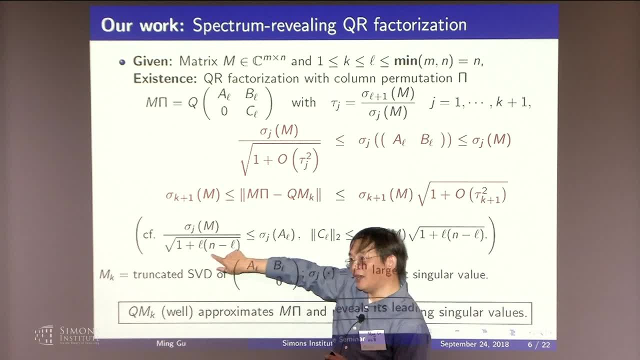 Right, This is a constant, Demand-dependent constant. You only get a fraction, But here you could expect to get a very accurate approximation. Excuse me, Could you give the intuition for why you keep the B around? Because your low rank approximation. 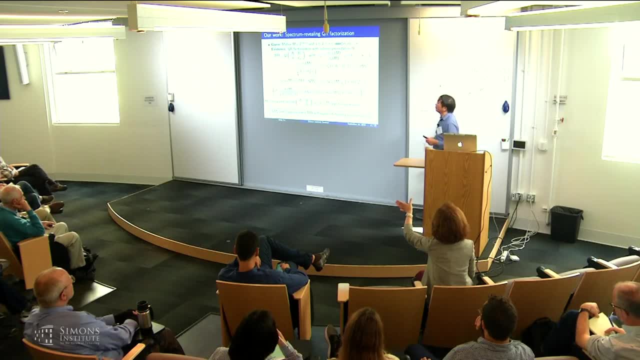 is going to be linear combinations of the first L columns of Q, right, Yeah. And what does the B help you? You already get that by having A there. If you only look at A right, that's only just the A. 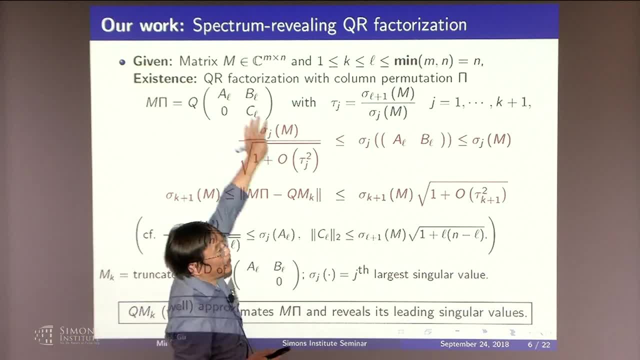 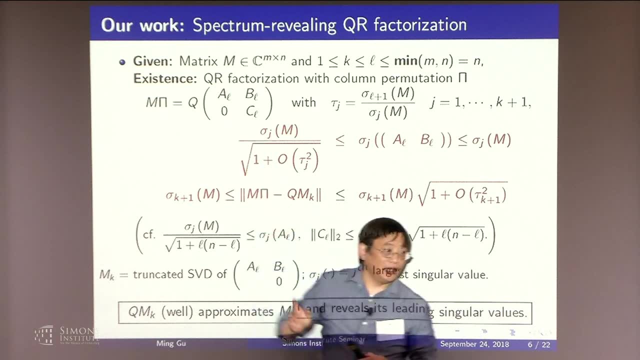 That's only L columns of matrix. The B actually represents the linear combination of the remaining columns into the leading columns. Oh, I see, Sorry. Okay, So this typically is good. I use this, I quoted this word well, because sometimes it's not that good. 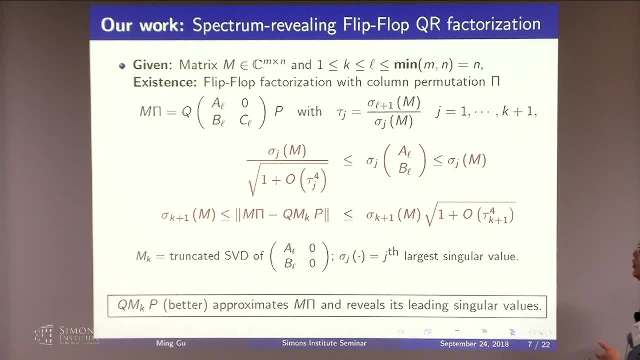 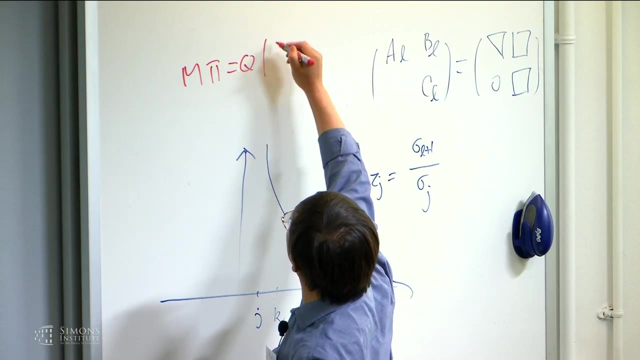 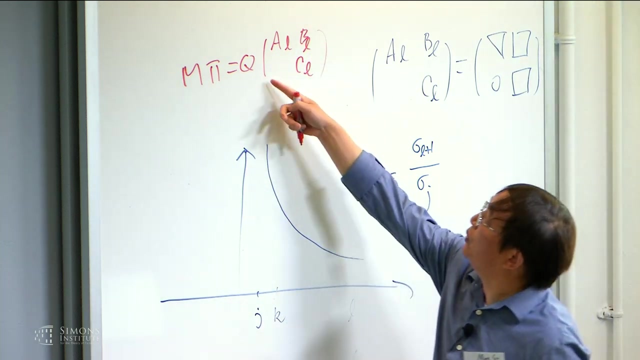 Okay. So if you want to do more than tau squared, you could get into tau to the fourth by doing the Stewart type approximation. So what is that? So you have M. pi equals Q. This is the typical Q-y factorization. But if you do, 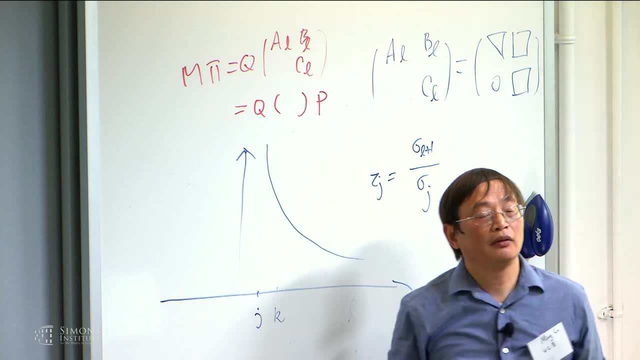 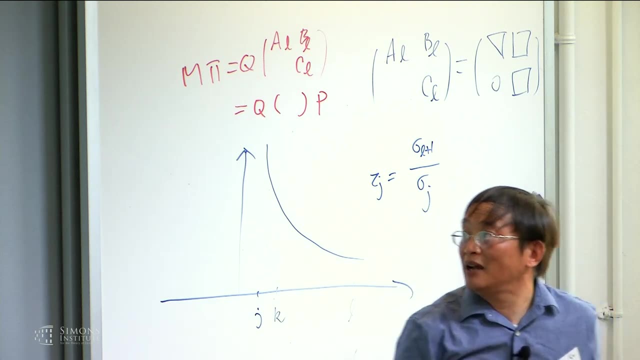 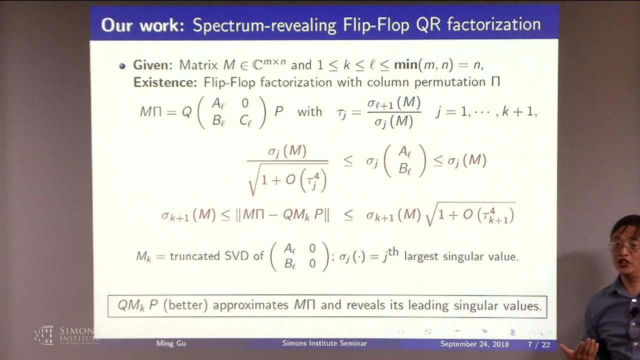 And Lp Factorization of this. This is up triangle. You flipped to lower triangle. If you do that, then you throw away this piece, the training piece. you get an even better approximation, Instead of the tau, to the two. 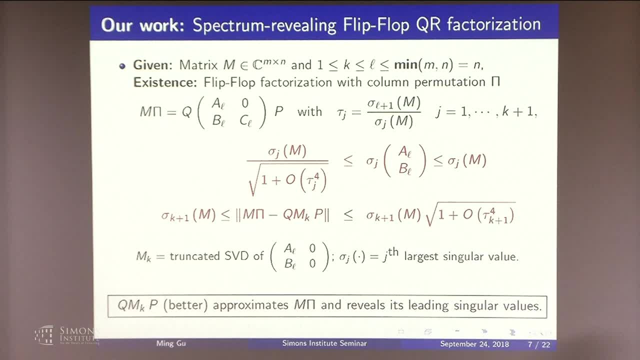 now it's tau to the four. Okay, And you would ask, you know this would cost much, right? In fact it doesn't cost very much. We're going to see some. Well, hopefully we'll see some numbers. 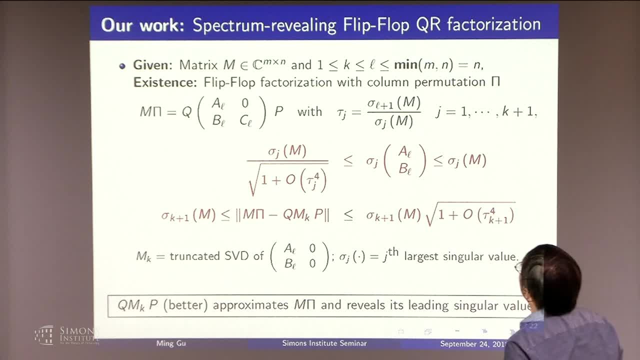 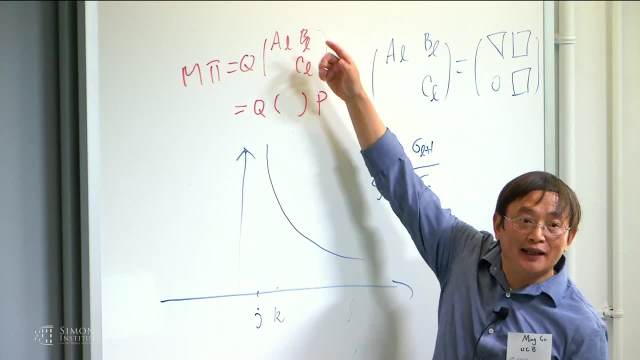 Could you say what P is, What the P is P? This is just the. You're doing an Lp factorization of this matrix. It's like the QR of the transpose of this matrix. The P would be an orthogonal matrix. 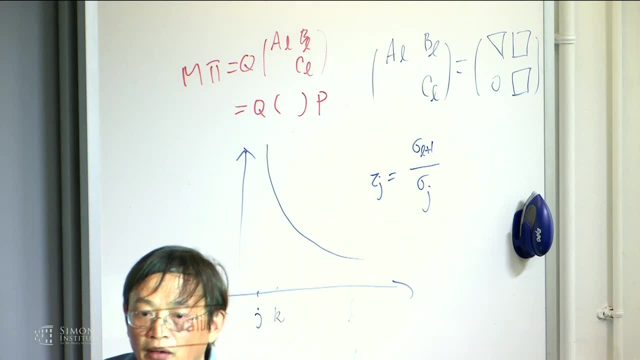 Okay, Here's Michael. You're missing some transposes there. How did B and C get on the A there? Oh, sorry, I was using the old note here, but this is a different thing. This is a lower triangular matrix. 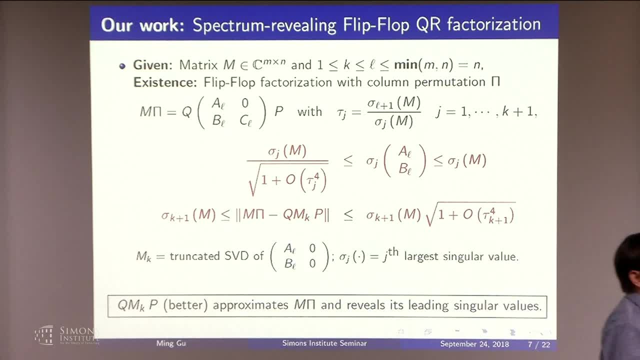 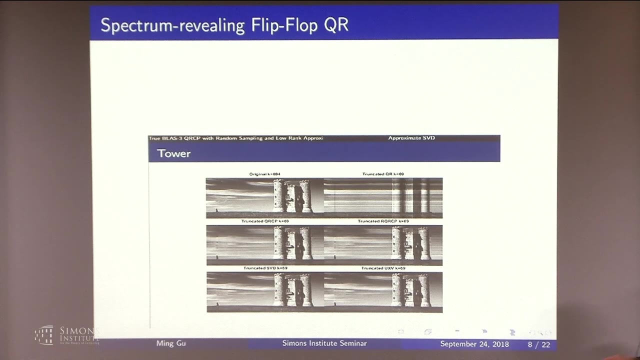 not upper triangular. Not the same. Yeah, not the same. Okay, Typically, you would do much better with this, Okay. So An example to see all the differences: here you have your tau. This is going to be 600 by 600 matrix. 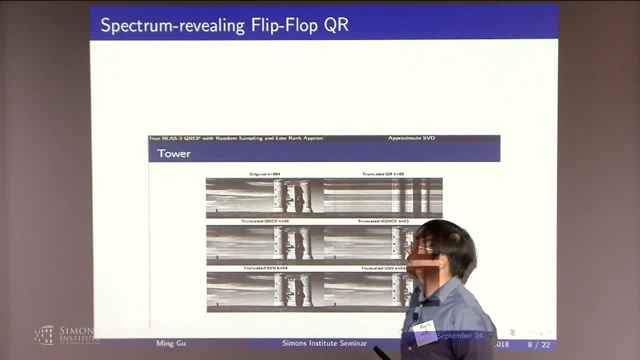 And if you do truncated QR with 60 steps without any column, you're going to get a matrix Column shuffling. this is what you get. You know you lose the whole picture If you do truncated QR with column pivoting with 60 steps. 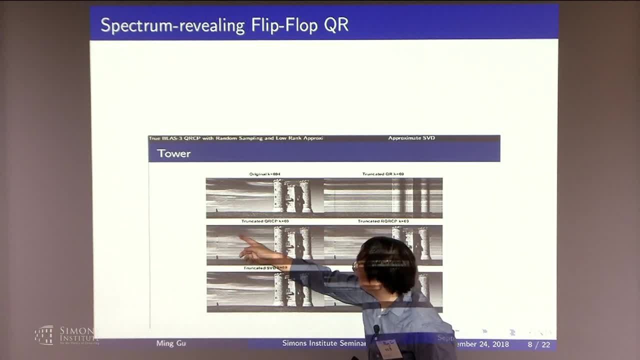 you get something like this: There's some smearing of the clouds, but you get something Okay. So typically if you do QR with column pivoting, it's a very slow operation, But if you do a randomized QR with column pivoting, 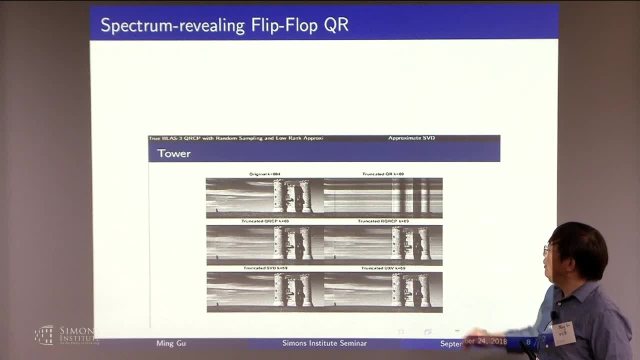 you will get a result that's as good numerically, but it will be at a fraction of the original speed And, as you can see, this randomized version looks just like this one, But still, you see some smearing If you do a truncated SVD. 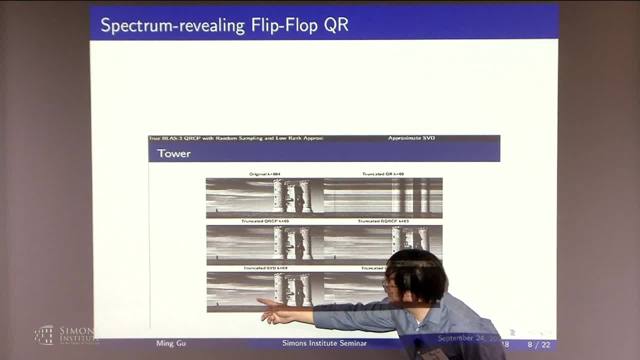 this would be again rank 60. And you can see that this picture looks very close to the original picture. You do lose something, but it looks to the eye. the difference is very small If you do what we call flip-flop. 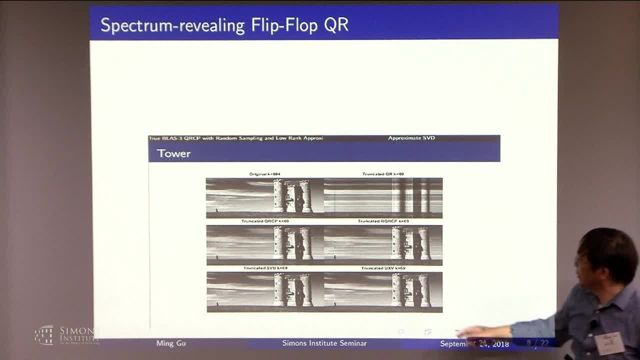 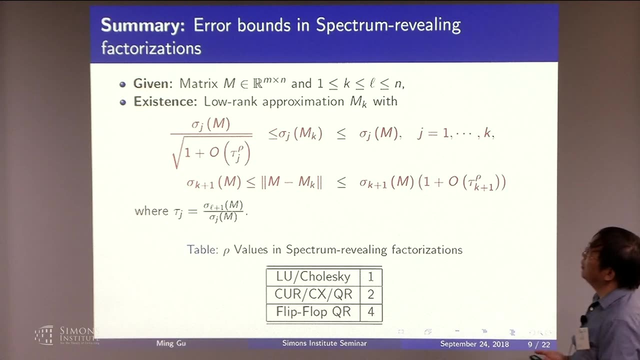 you know, you do the QR and then you do the LQ. this thing looks almost the same as this. The difference is tiny. You probably don't see the difference with the eye. Okay, So we've done a lot of different factorizations here. 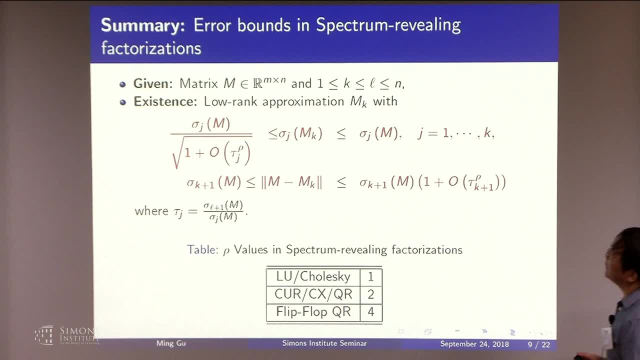 This is just a summary of what we have done so far, And it turns out that for all the major matrix factorizations, you can do the spectrum-revealing version of it, And I'm going to skip all the details, but you can compute these factorizations efficiently as well. 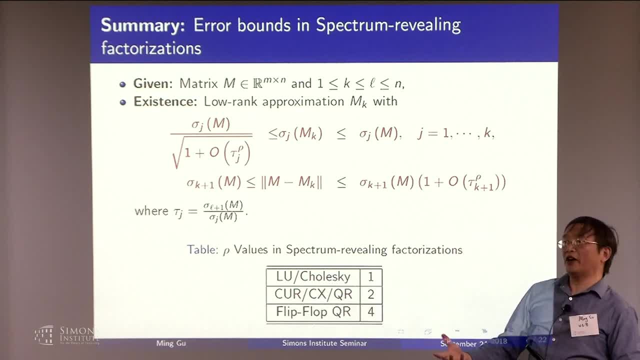 So typically we have the ALU factorization, we have the Cholesky factorization, we have the QR factorization And the CUR and the CX. these are the inventions of these similar organizers, But all of these you can get these bounds. 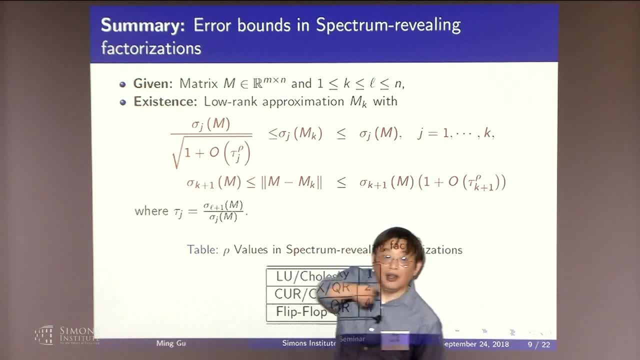 The only difference is in this tau value. So if you do QR, this tau value is 2.. If you do this flip-flop QR, this value of tau is 4.. But if you do ALU or Cholesky it's 1.. 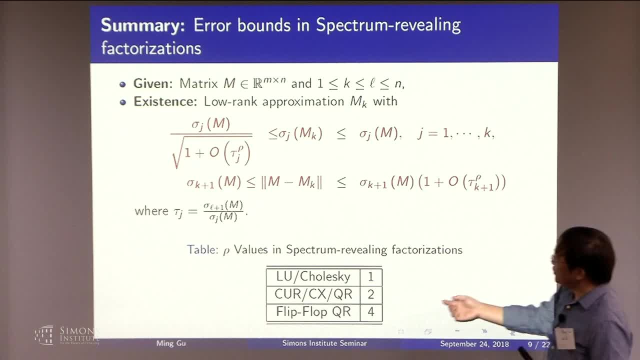 So it's much less accurate. If you do CX or CUR, they're just as accurate as QR. I probably missed a little bit of context on the image factorization you did on the previous slide. Yeah, Is this. are you storing the? 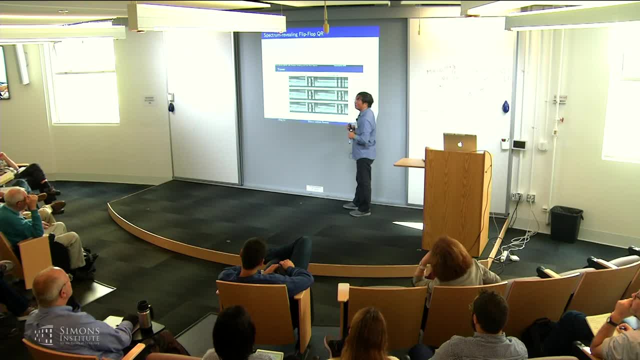 is your matrix? just every, is every entry of your matrix just the one pixel of the image? or, Yeah, the grayscale, Yeah, It's the grayscale of the image. So your rows are literally the rows of your image. your column are literally the column of your image. 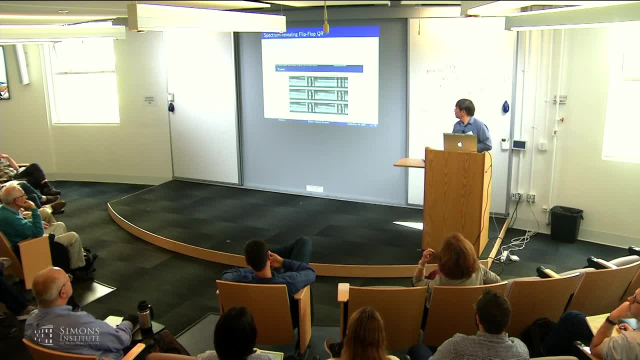 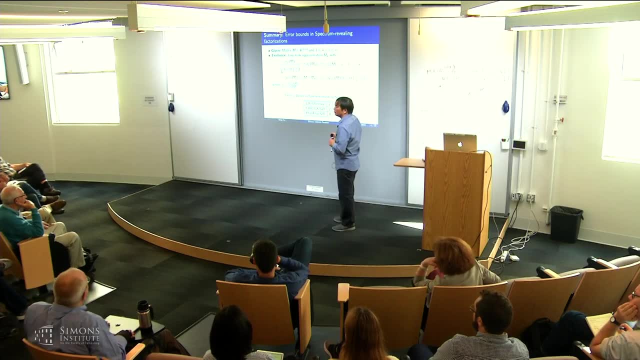 Yeah For these types of spectrum-revealing factorizations like: are your pivoting rules the same as they are if you are using different pivoting rules, For example for the ALU right? it's basically like an ALU with column pivoting. 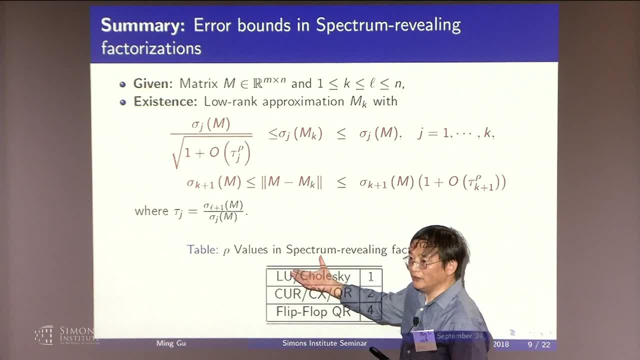 I mean with complete pivoting, But we have a way to compute this quickly. Typically you don't do this right. It's supposed to be slow. but if you do randomization you can do this very quickly. And the same thing with Cholesky. 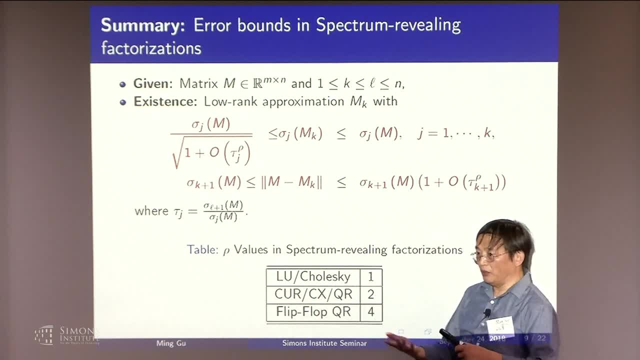 or even with the CUR CX factorizations, you have a way to pick the column pivots very quickly. Flip-flop QR. does that correspond to one step of the Francis QR algorithm for computing eigenvalues? It's basically, you can think of this. 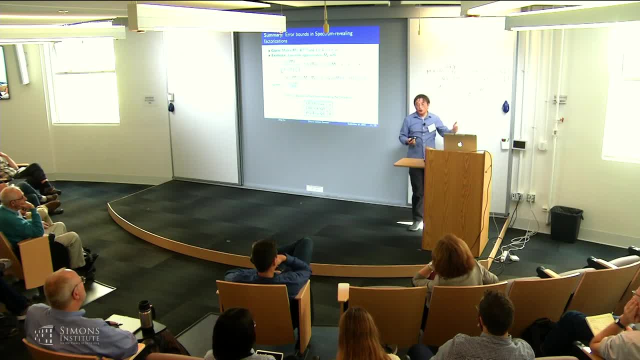 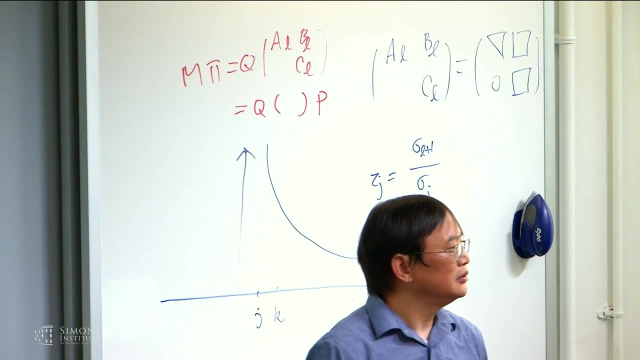 as like a subsequent iteration on the whole matrix. It's also the Stewart's method. Stewart called it a P or Q or something: QLP, QLP. yes, That's the Stewart QLP algorithm. Yeah, but he does it very slowly. 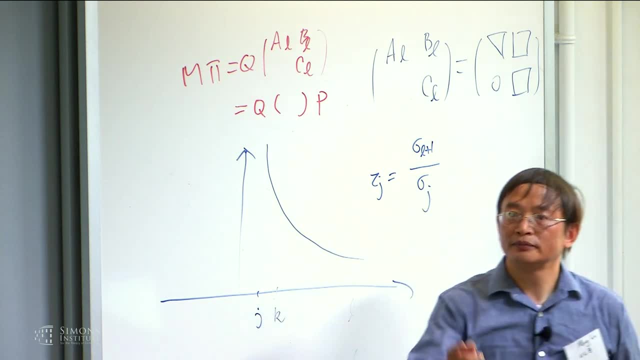 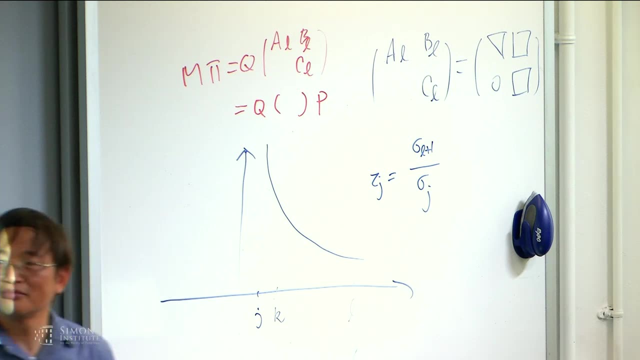 We do it very quickly. So for the Cholesky, do you mean that it is only applicable to the case when M is real, symmetric or Hermitian? Oh yes, of course. Okay, and you have only rho equals to one. 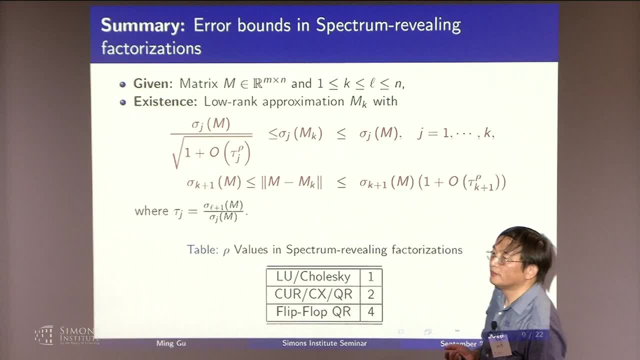 Okay, yeah, For Cholesky it would be diagonal pivoting. Is there any way to improve the performance of a Cholesky, to have a higher order? The question is, can you do this better than this, right, Yeah, yeah. 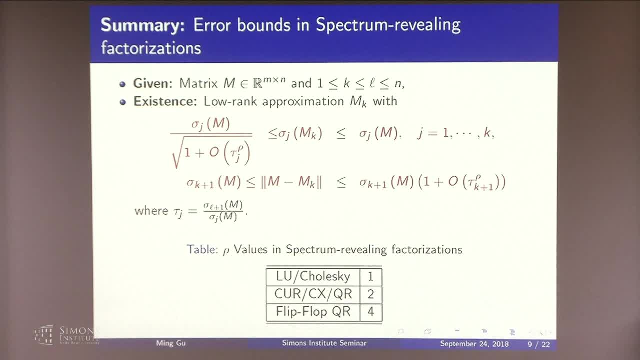 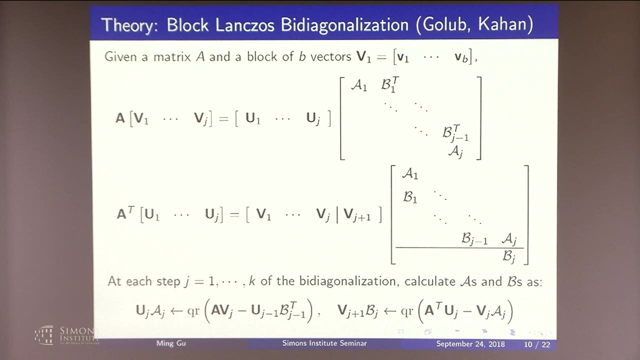 You can If you really want to work through it. there's better ways to do it. Yeah, Okay, So those are based on matrix factorizations. As you saw, the best you could do was for a tall value of four. Most of the time, this is good. 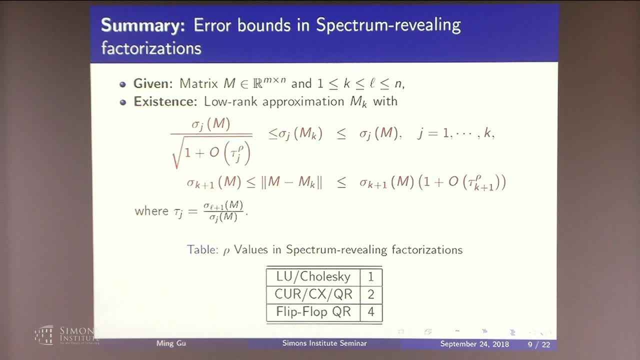 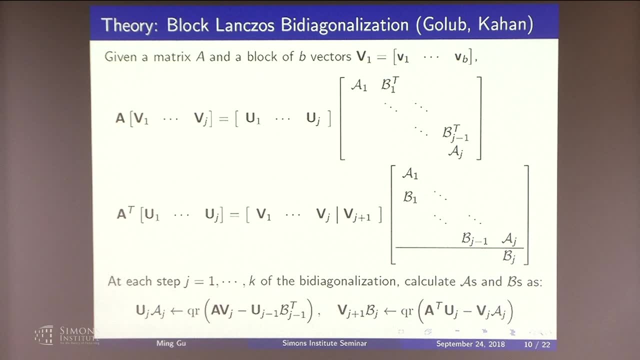 but sometimes you think this is not enough. You want to do better than this. If you really want to get a high-quality lowering approximation, you've got to do block line shots or block bilinearization, And this is the math for it. 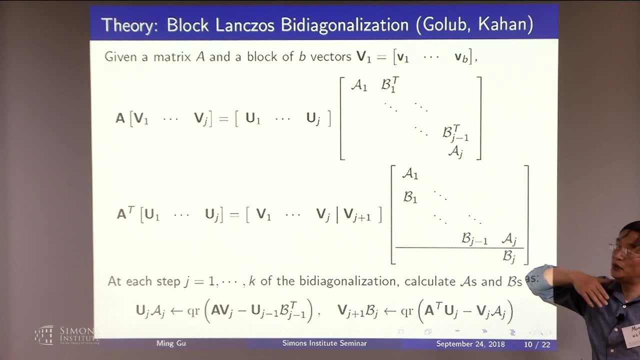 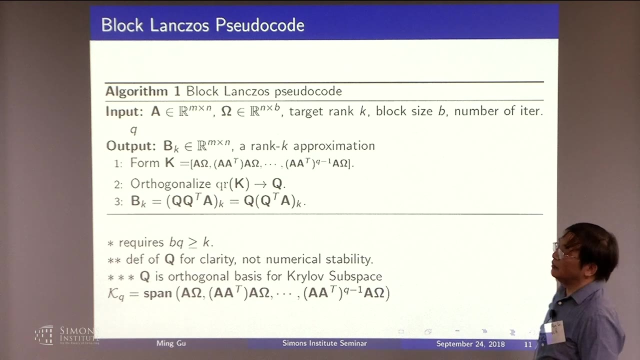 You're given this V1 matrix, initial matrix, with B columns, and you just do this bi-diagonalization standard thing, Okay, so the details don't matter for us at this point. So if you kind of come up with a mathematically equivalent, 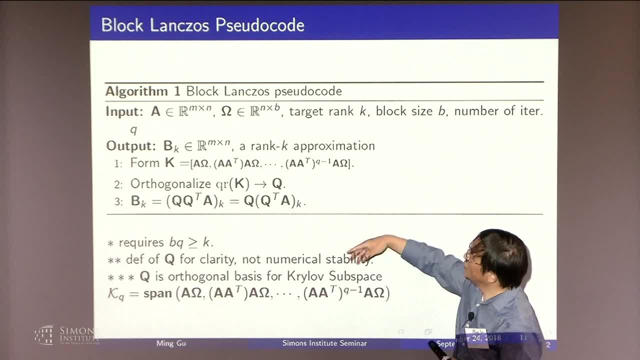 but easier to understand version of this. this is what it is. You're basically calculating the orthogonal space, orthogonal basis of this subspace, columns of this matrix K. You don't calculate it this way, but mathematically this is what it is. 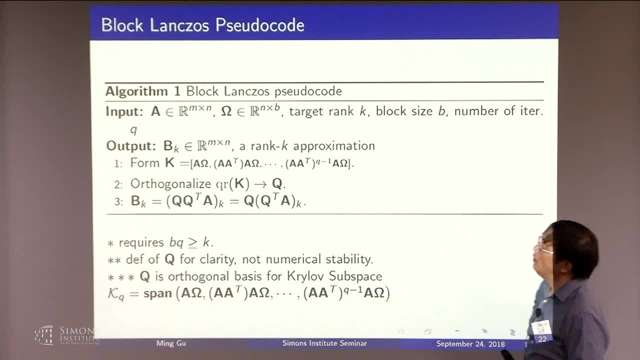 You get the basis for this matrix and then you do truncated SVD. So there's a few things to be said. The B is the number of columns in your omega, which is the initial matrix, And you're looking for a rank K approximation. 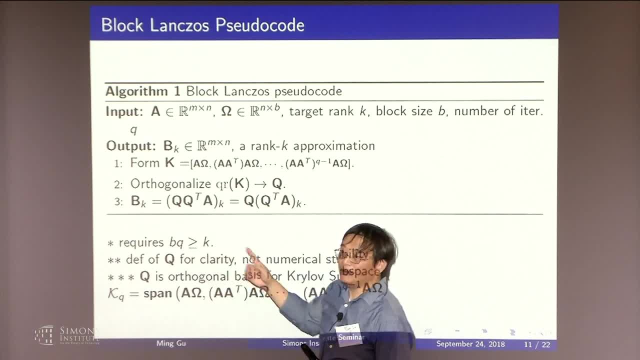 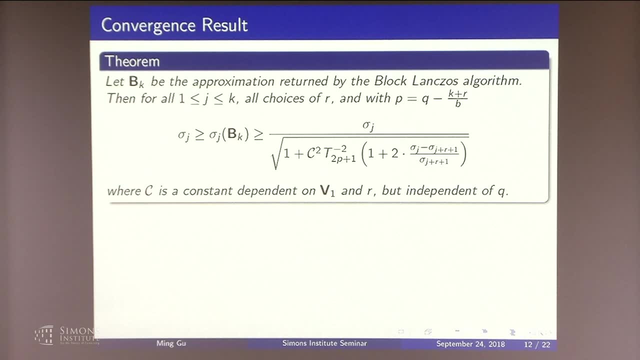 So B times Q, Q is the number of steps. That needs to be bigger than K. That's the only thing that you require for this to work in theory, So I'm going to just put the result right here. It looks very messy. 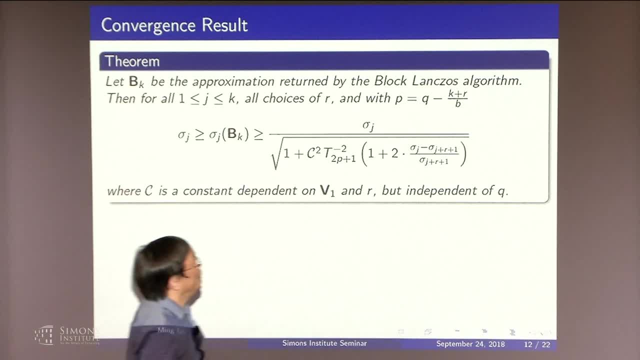 So what we're looking at is maybe the projection, the BK, out of the block Lanchard's algorithm, even though Lanchard's really did not do this work in particular. So you're looking for a rank K approximation. You've done Q steps. 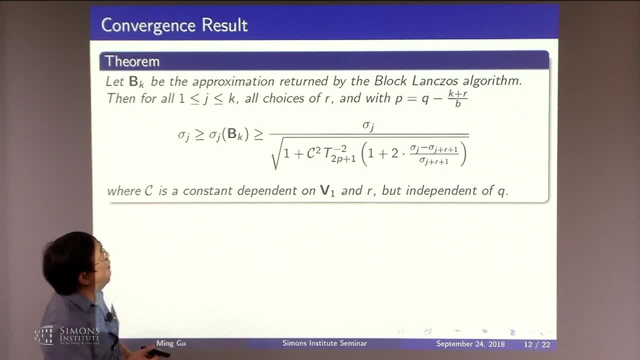 So there's a lot of parameters floating around, But the Q is the number of steps, B is the block size, K is the rank you're looking for. Here we introduce another thing called R. This R has nothing to do with the algorithm. 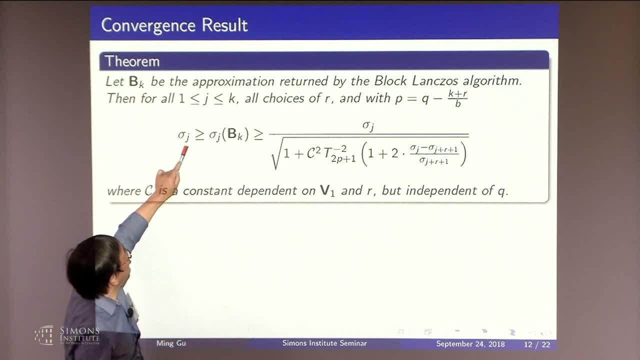 It's only part of our analysis. So you're looking at the j-th single value of this matrix. Then you can show that you get at least some kind of fraction of the true j-th single value, And the fraction is going to be one plus. 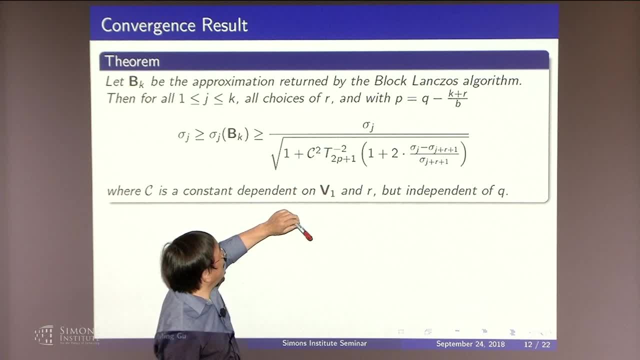 of course, something which hopefully will become zero in the end. The C is a constant. That's a messy, messy constant. We're going to ignore the details, But what's important is that, the way this is structured, the C does not depend on P or the Q. 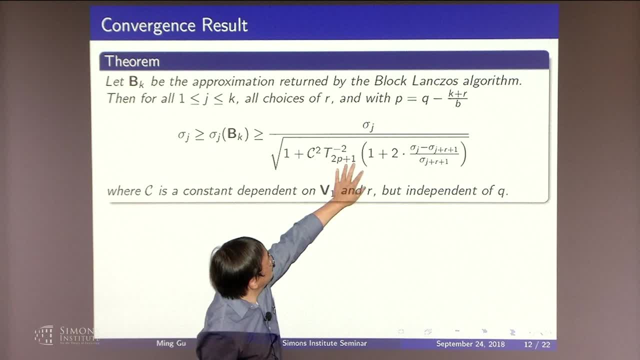 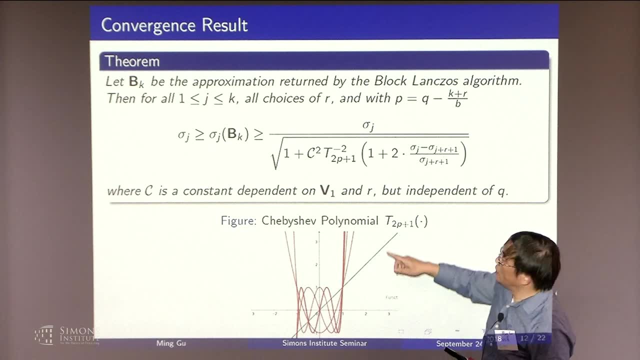 And this part of it is the chapter polynomial. So the convergence depends on this weird, weird thing. Ignore the details, But the point of the chapter polynomial is that this argument is beyond one Here. Then the chapter polynomial shoots to infinity very quickly. 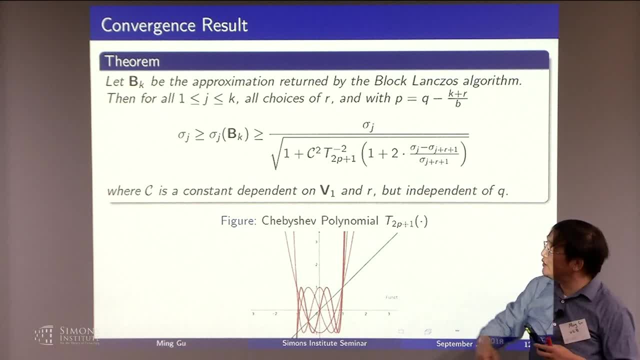 So as long as this is bigger than zero, you hope that when you increase P, this whole thing becomes zero quickly. Yes, So where is omega in this formula? Where is what Omega? Omega is part of the C. That's the initial matrix. 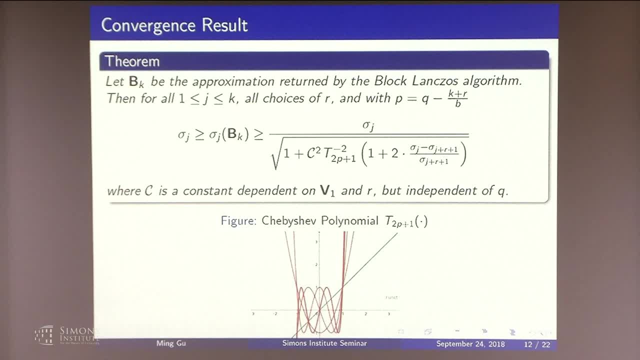 OK, What is capital T? Capital T, Capital T- That's the chapter, polynomial, OK. So the thing is very messy, It's very hard for the eye to digest in a few seconds. But there's R here which is not part of the algorithm. 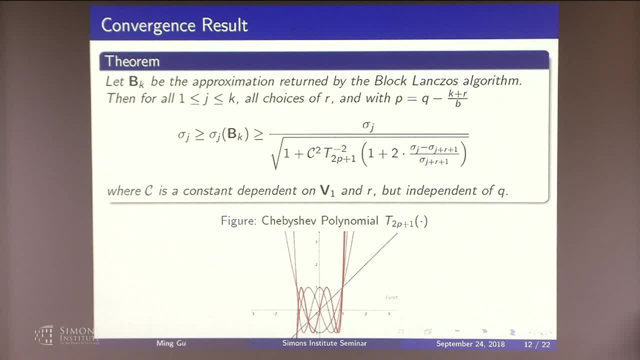 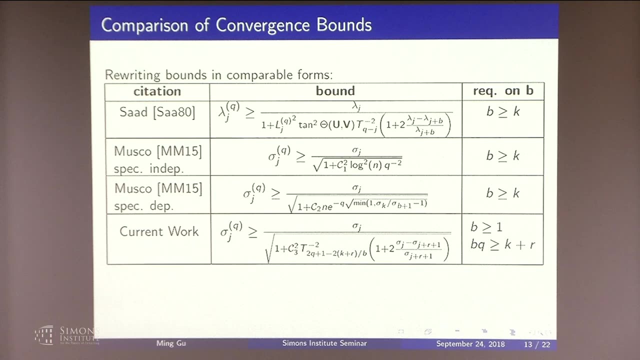 It's some artificial parameter that we introduced, And this is what it is. So the question is: what do you do with this? OK, Before we see what we do with this, let's just do comparison with what people have found so far. 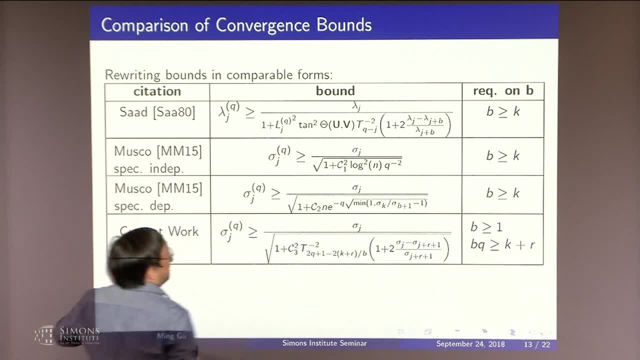 So Saad was the one who was the one who started block line choice. This was in the 80s. He had a bound like this. This lambda could be thought of as sigma squared And Moscow. this is like three years ago. 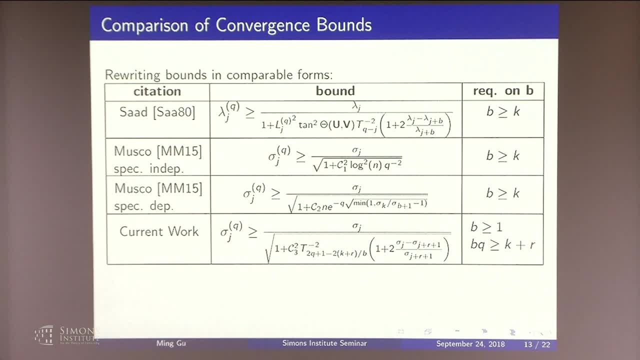 they had a very interesting paper that was for independent lower bound. In the form that we're looking at, probably it's something like this: There's some constants, and then you have Q negative 2. And the Q is the number of iterations. 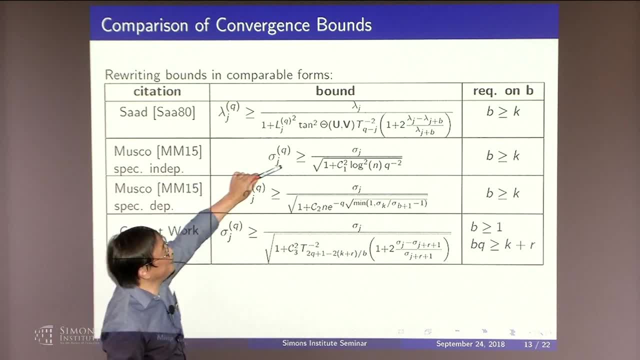 So essentially the idea is that you would eventually get convergence in the middle of the gap. No matter what back gap is, no matter what happens to this curve, you will get convergence. But numerically this does not give you very much because your Q never exceeds N. 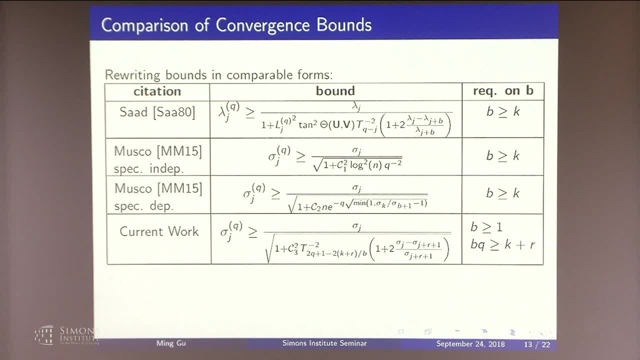 So all it says is that you get a fraction And you could introduce the gaps, but that would be kind of similar to what we would see in a tritoneal bound. So our bound is very messy And it has this artificial parameter r in it. 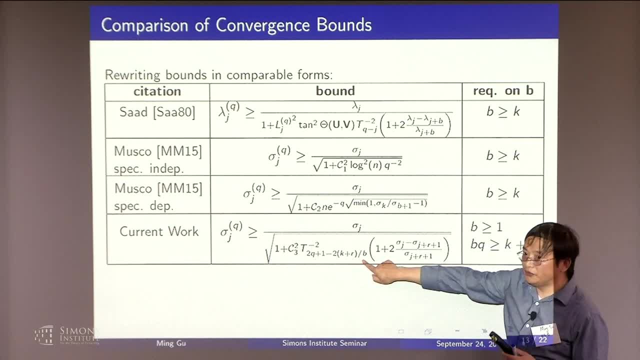 The r goes into the degree of the chapter polynomial, but also into the argument. So the bigger the r, the smaller the degree, the bigger the argument. So there's a balance. Yes, Do you need the gap here? Yeah, There's a gap. 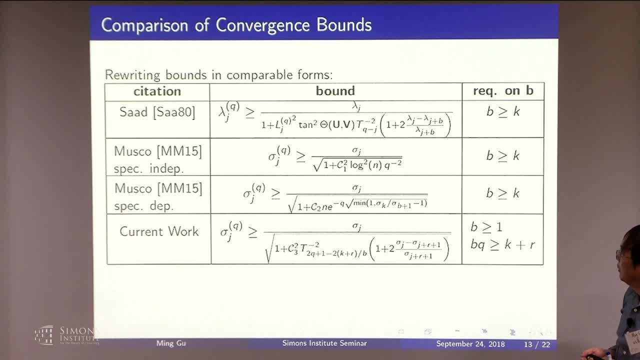 So vr, that's what it controls, right, The gap. But why do you need the gap? It's just a low rank approximation, There's no gap. So can this be 0? So here, what you know is that when you increase r. 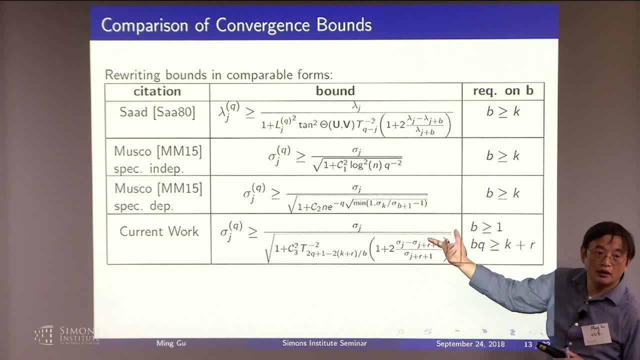 this ratio, this guy is bigger than this guy. So what happens if they're equal? What happens if all the trains are equal? What happens if they're all equal? right For this argument, we're going to ignore the case that they are all the same. 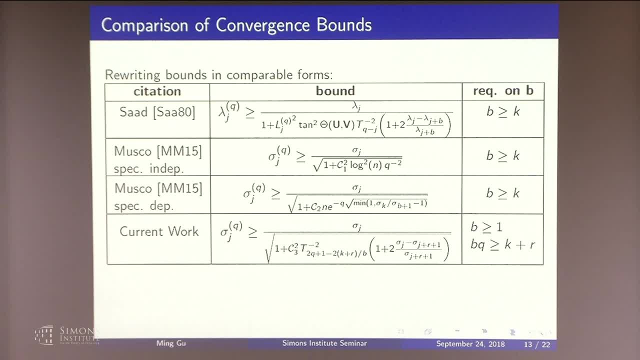 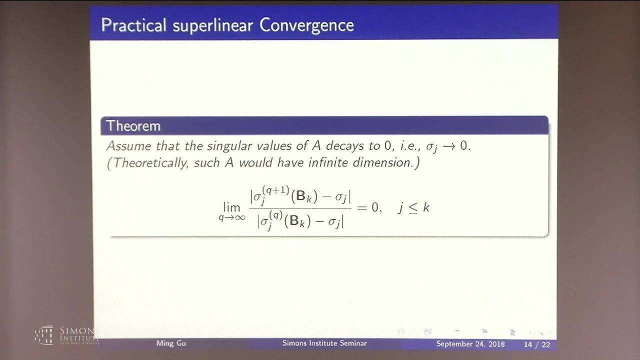 Because if they're all the same, you have to ignore some of those things. Your method will not recover those. The multiplicity has to be smaller than the block size. OK, here's the punchline. It turns out that if you play with the r value correctly, 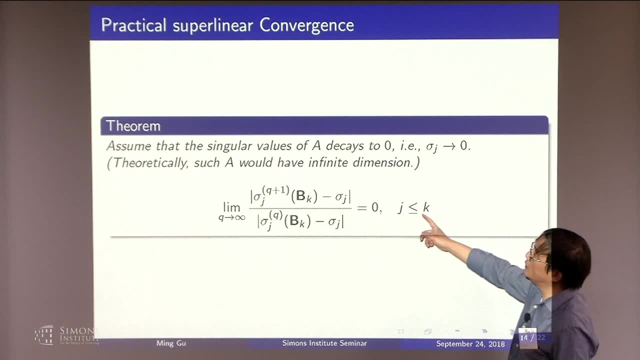 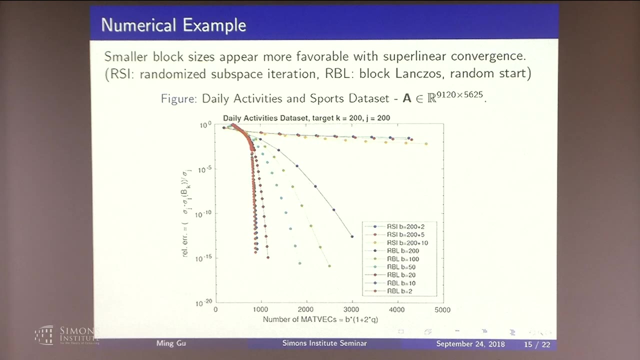 we can show that the bound we showed implies superlinear convergence. So that is, if you pretend that your matrix has infinite dimensions, your sigma is converged to 0, then you have this thing. What's this thing? So you can see it from this plot. 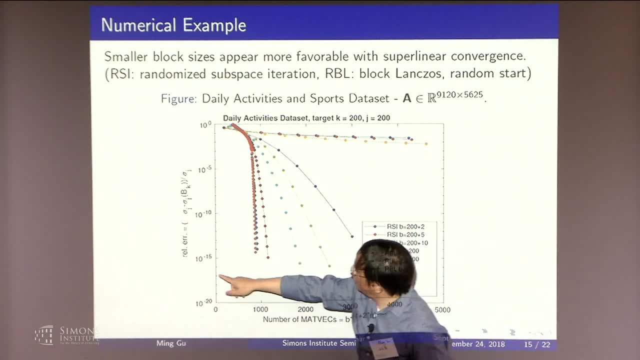 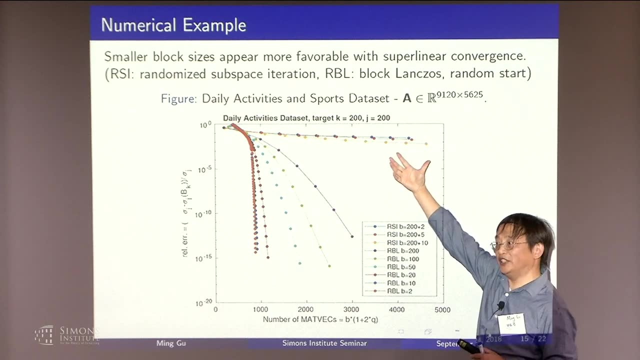 You're looking at the convergence of the 200th single value. OK, and this is with randomized subset iteration, which is known to you. It's known to be a linear convergent method And this is block line shows with different block sizes. 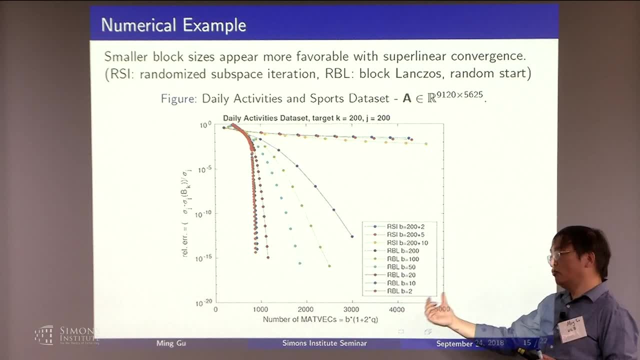 And the vertical horizontal axis is the number of MACVACs, the number of matrix vector multipliers. That's the work that you have done for computing the single values. As you can see that these all show superlinear convergence behavior. The bigger the block size, the slower the convergence. 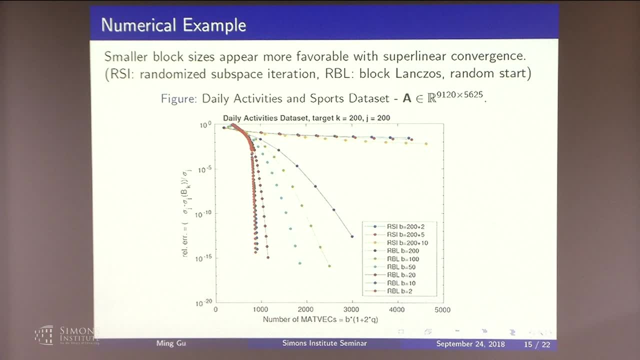 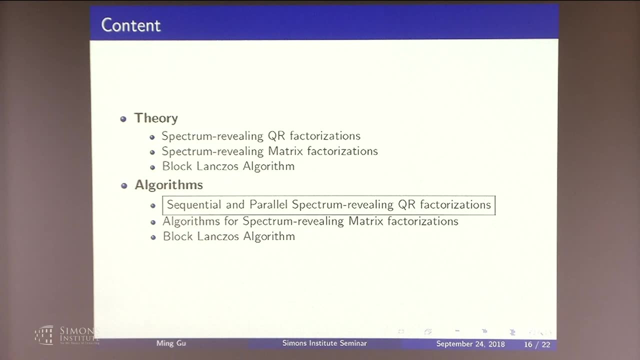 But still they are superlinear, convergent, OK. so how much time do I have? Five minutes, Five minutes, OK. so I'm going to jump into the algorithm part. I only have five minutes, so I get to show you a few plots. 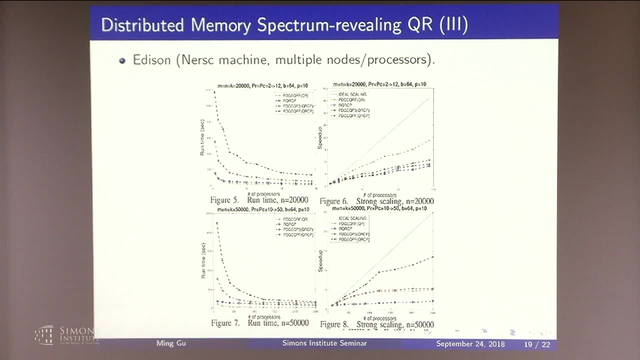 I'm going to skip these and just do this. So this is distributed memory implementation of the spectrum-revealing QR. So what you see here is a 20,000 by 20,000 matrix, And here we take the rank to be 20,000 as well. 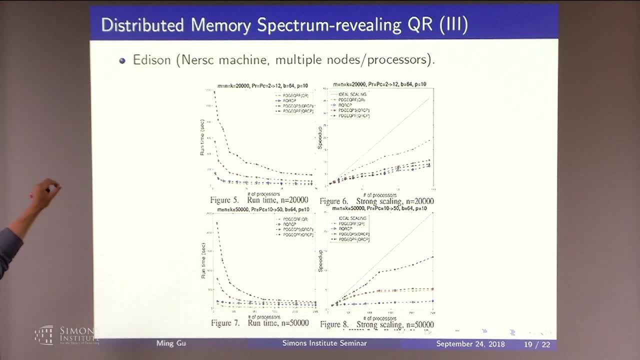 So the layout is that we have the same number of rows. It's a square layout. PR is the number of processes And PC is the number of processes as well. So you have a square layout of the processes And the block size is 64.. 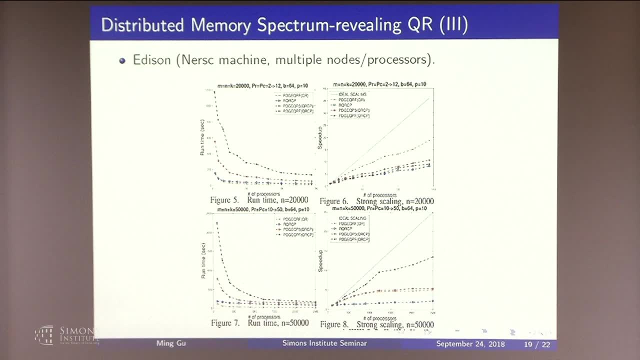 The P is 10.. You can think of this as some kind of L-related parameter in this calculation, And so this is the runtime plot. So we have looked at a number of different implementations. So there's the LPAC implementation, a scalar pack implementation and also a scalar pack. 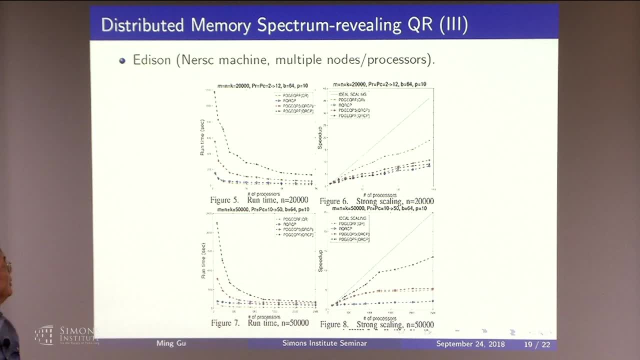 maybe future scalar pack implementation or something. It's supposed to be faster than the QR with the column pivoting And this is our implementation. somewhere There's also the QR without column pivoting. That's the baseline comparison. So this is our algorithm. 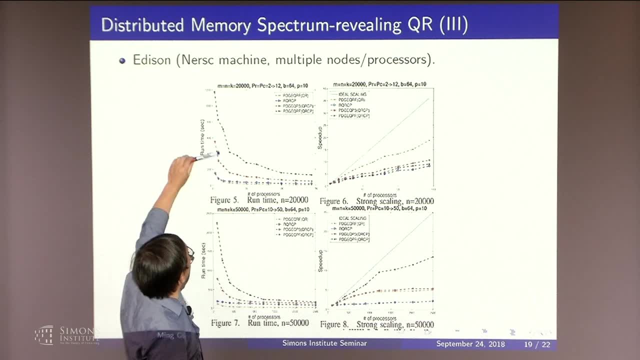 This is the QR without any column pivoting And these are some other scalar pack implementations with column pivoting. You can see that we have a huge speedup over these things. And this is the strong scaling of these algorithms. They don't scale very well. 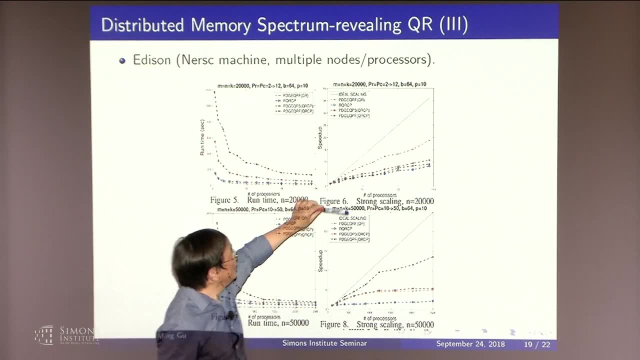 That's because, for the size, 20,000 by 20,000, by the time you have a lot of processes. each process has very little work to do, So that's why there's no good strong scaling. But the big thing is that when you start, 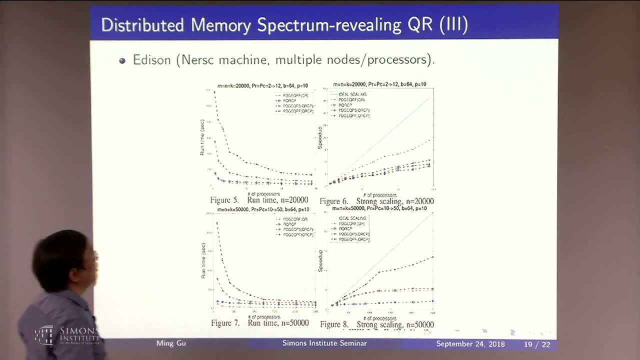 we are much faster than the other methods And this is the same thing as before, except that the demand is much bigger. This is 50,000 into 20,000.. You see, the same kind of behavior. Are those random matrices? 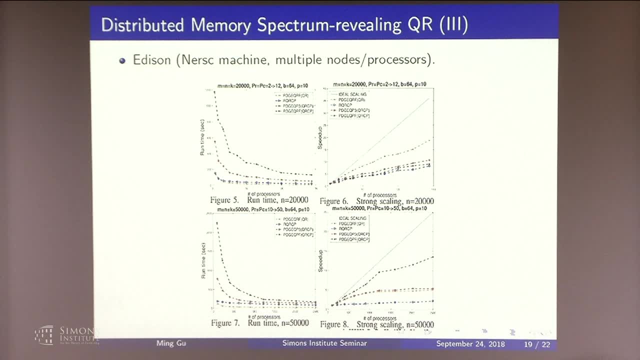 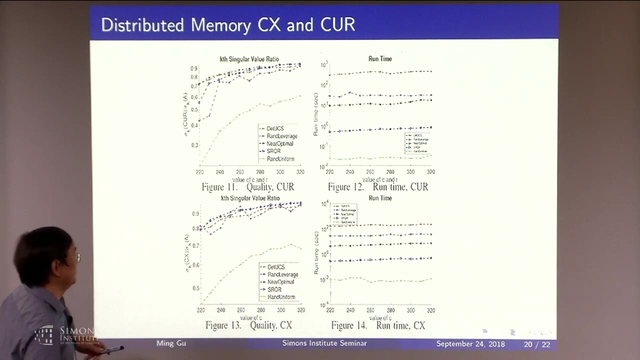 These are random matrices. yes, Gaussian random matrices, Uniform random matrices, Maybe, because here we're just going through all the way to the end, so it makes little difference. This is CX and the CUR. This is CUR, This is CX. 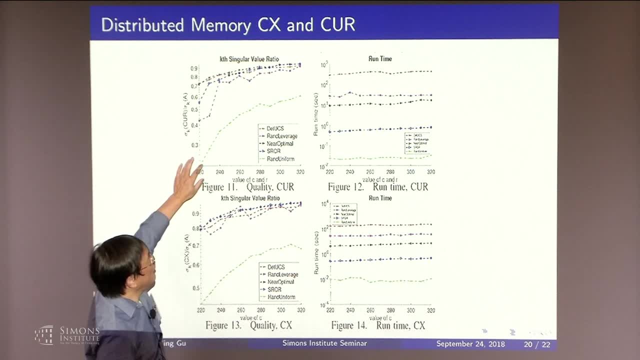 So here what we're looking at is quality versus time. Quality means the ratio between the computed J-th string values versus the original J-th string value. So if your ratio is 1, that means you have captured the string value correctly. If it's less than 1,. if it's much less than 1,. 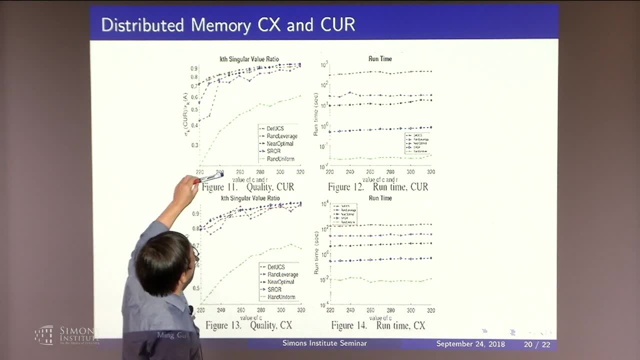 you have not captured it correctly. So this is our method somewhere here Against a random method, random commutation and some other competing methods. As you can see, if you don't pivot correctly you don't get much. But for us, if we pivot correctly, 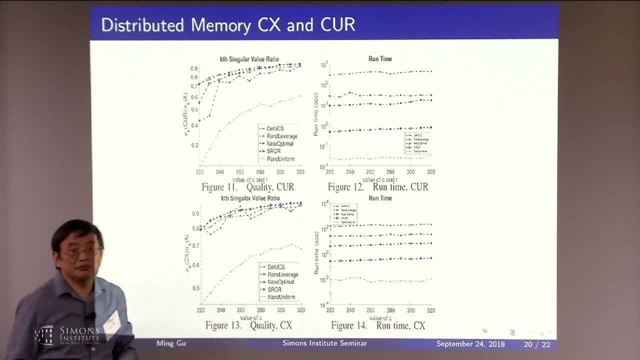 as you increase the rank, your ratios become very close to 1.. But not 1,, which means that this is not really. if you are looking for high-accuracy approximation, this is not very good. Front time: This is QR with random pivoting. 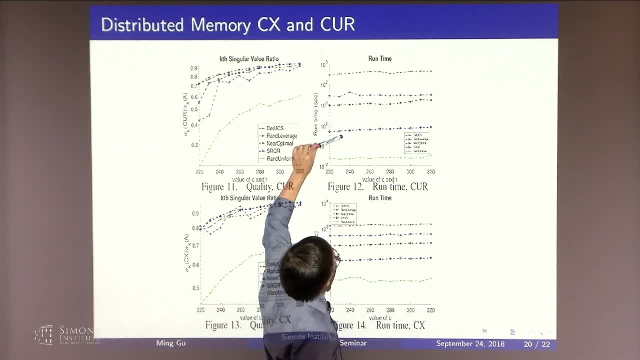 This is our method. These are the competing methods. We are effective 10 or better than the other methods. That's the CUR. This is CX. It's kind of the same kind of behavior. This is random column permutation. This is our method. somewhere. 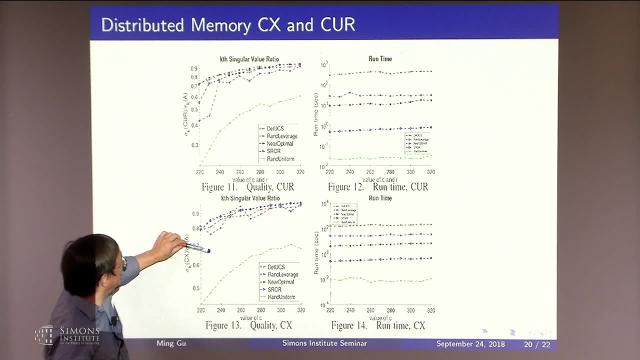 And these are the competing methods. So for the competing methods and our method the quantities are compatible, But our method is here. as far as long-term goes, It's again maybe effective 10 or more better. Thank you very much. 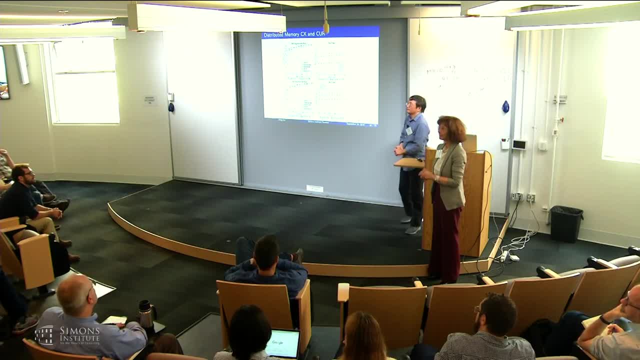 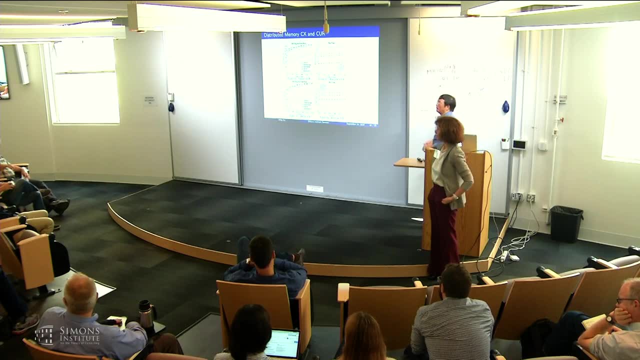 There are questions for me. Do you have a sense of like your bound depends very much on the block size in this sort of like complicated way? Do you have a sense of like how you should choose the block size? 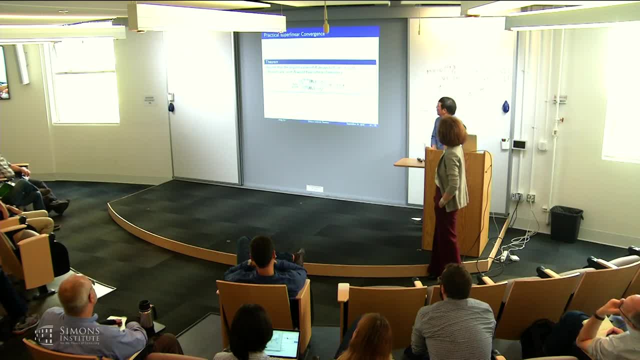 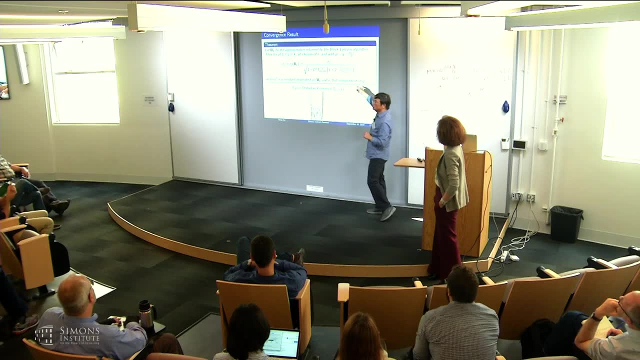 Should you just like try a bunch of different ones and see which converges faster? Or like This one, B versus Q, Like you have B and Q and Yeah, you have like block size This one. 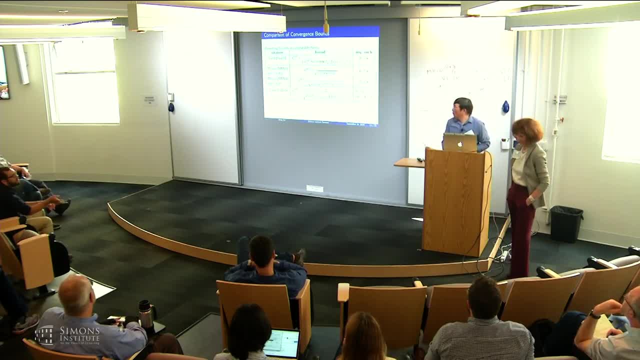 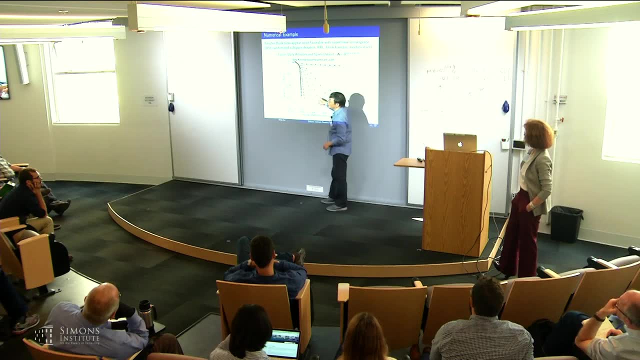 Yeah, OK. So I know the R doesn't factor in the implementation, but the B would be in the implementation, OK, So as-wise commutations go: The smaller the block size, the better. Right, So this is: B equals 1.. 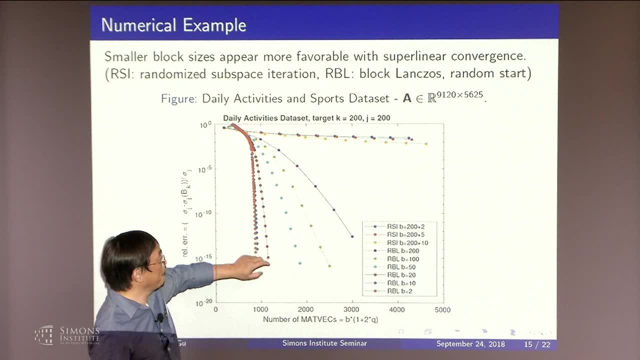 This is 2.. This is, I think, 4., And so on and so forth. So, as-wise convergent speed goes, Smaller block size is better, But on the other hand, performance depends on bigger block size. 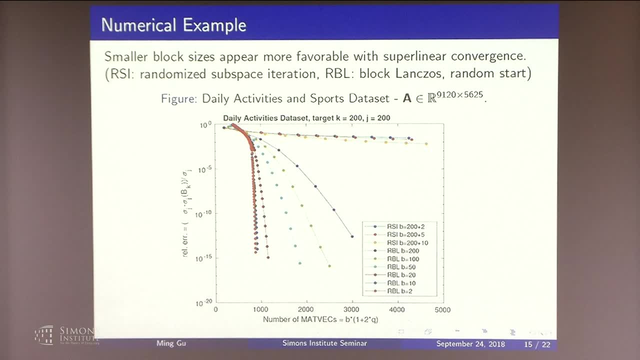 So this plot by itself does not tell you which B value is better, But our experiment seems to suggest that B equals 1 is better, B equals 1.. Because B equals 1 allows much easier handling of deflation or that kind of stuff. 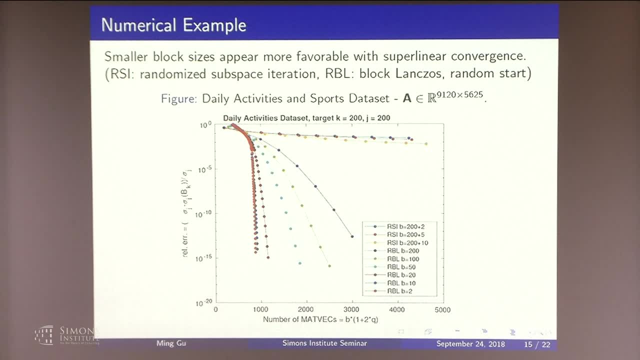 If your B is bigger than 1.. But it might not be the right choice because it's like slower, because you don't get the beads from multiplying over and over. That's right, But then there's a lot of other issues that would become so much simpler. 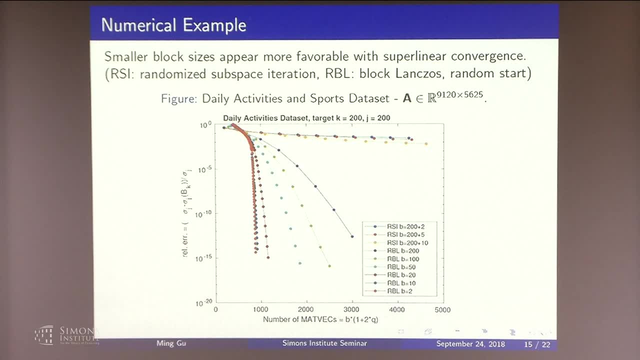 when B is 1.. Another question: Yes, Sorry, I was wondering about the sort of any vision behind going from top to the 2 to the bottom. Is there a way to do that? Is there a way to do that? 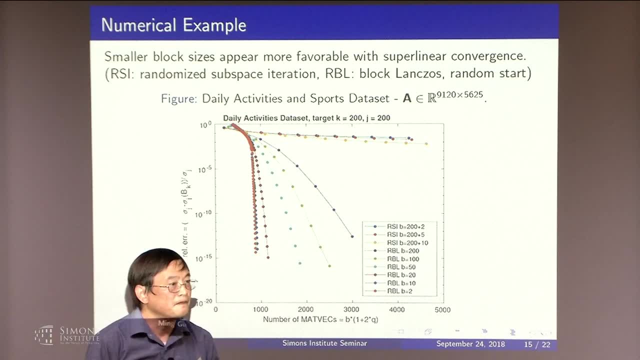 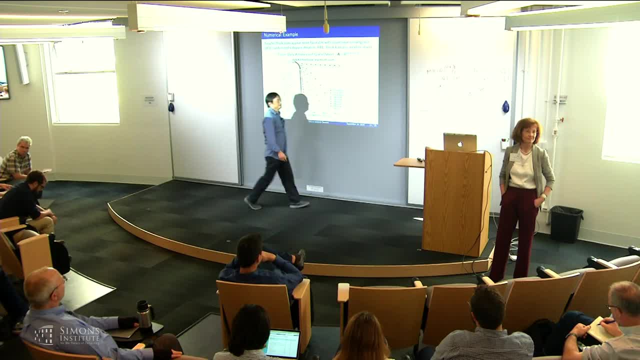 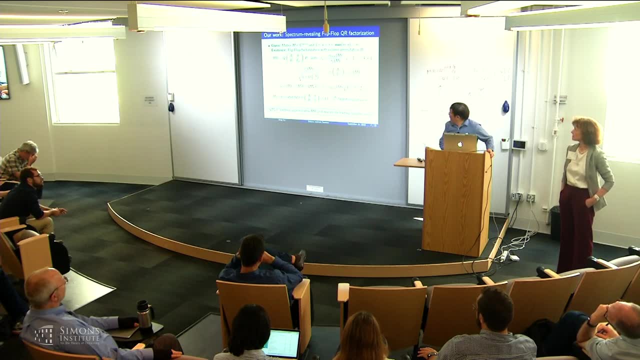 to the top, to the 4, and sort of whether you're missing like a uniqueness thing here or is it possible to sort of to iterate more? and So this is the slide you're talking about, right Or run before, maybe like 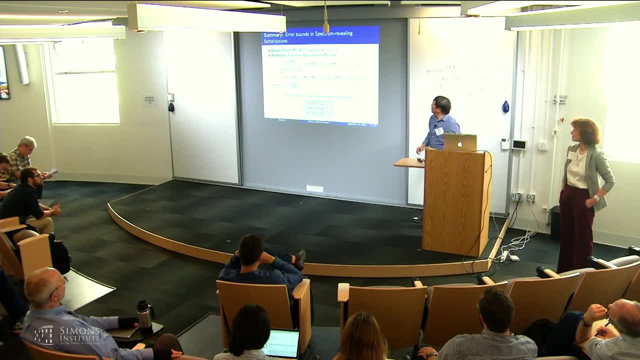 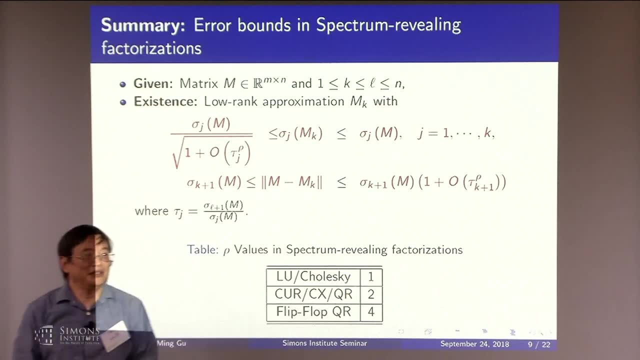 Okay, yeah, So this is where the value is. This is actually I use the rule value here. If you do AOU right, Like I mean, it's so simple- you probably should expect to run it. You don't want to lose. 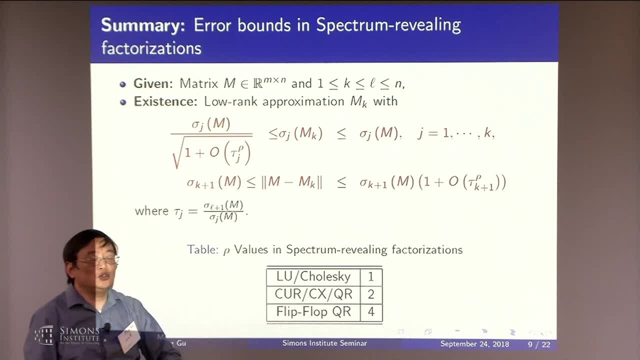 a lot of accuracy. But the problem for AOU, the only reason you do it- is because your L and U probably would be spots. My question is about 3-plot QR. Yes, So you do QR. you get tau to the 2,. 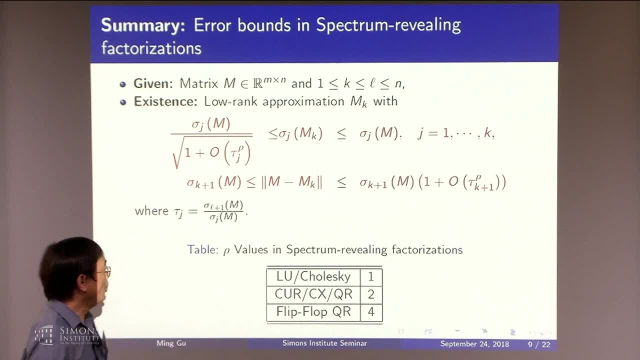 then you do another sort of LP and you get tau to the 4.. And I'm wondering- maybe I'm missing a uniqueness condition sort of property here, but is it possible that you do a QR again and get tau to the 6? 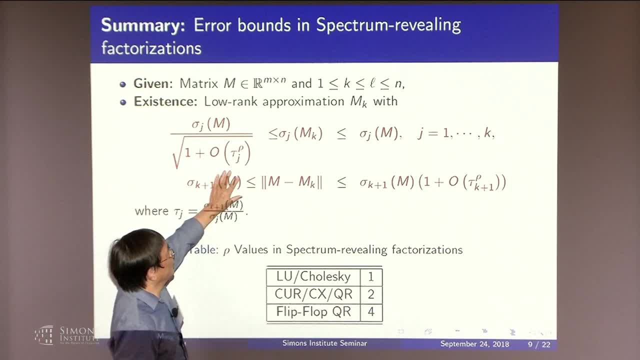 or something like that. It's just like intuition. So I don't know what you mean by uniqueness, because by the time you're doing this, you're just doing an approximation, Right? So by the time you do this, 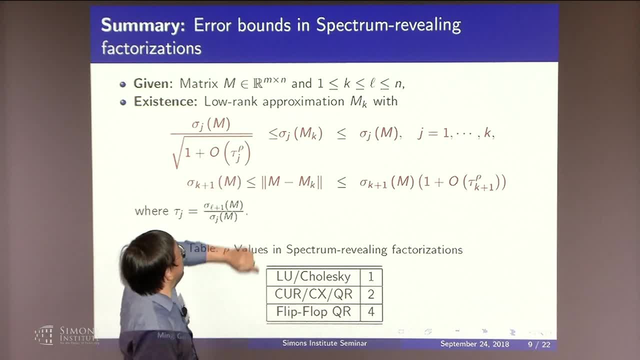 then this, the column permitting itself, is not going to be very important, So you can continue doing this, but this amounts to subspace iteration, which I already said in this plot. So if you're really into convergence, if you want to have